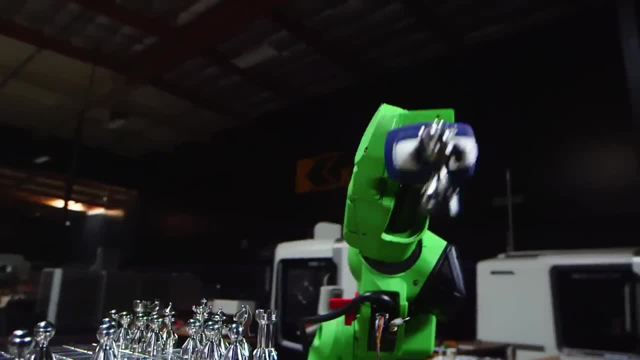 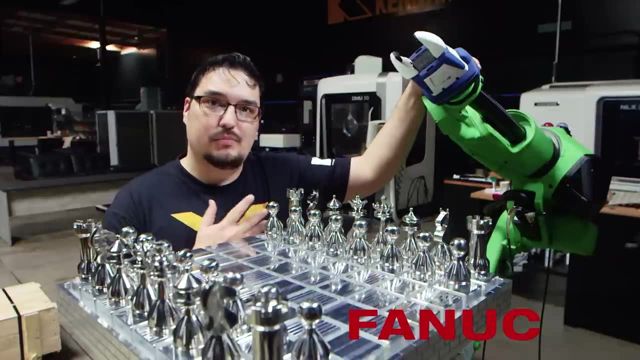 Not only that, the exact move that I used to beat my dad in two turns. Before we get started, I'd just like to say that this robot here is just like any other machine that we have in the shop. You need somebody to program it. 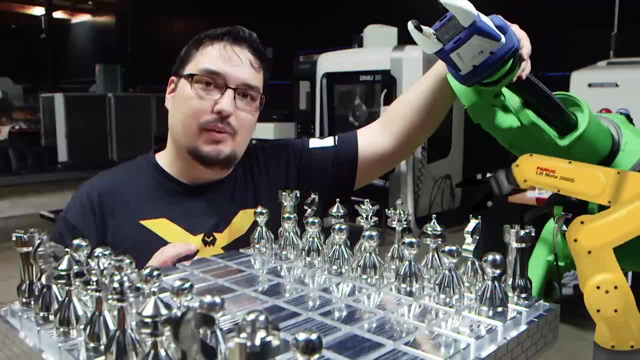 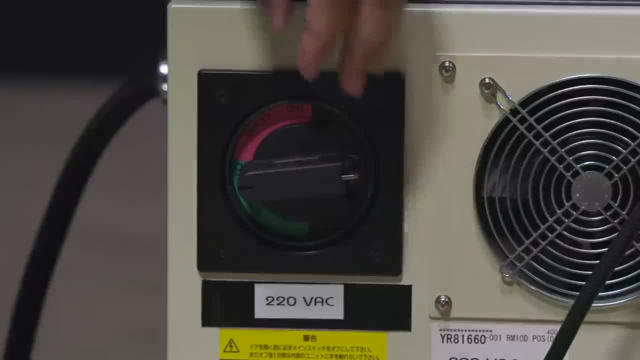 And it'll do exactly what you tell it to do. Today, I'm here to show you how easy it is to program a simple move like this. Let's start by going through all the steps, starting with step number one: how to turn on the machine. 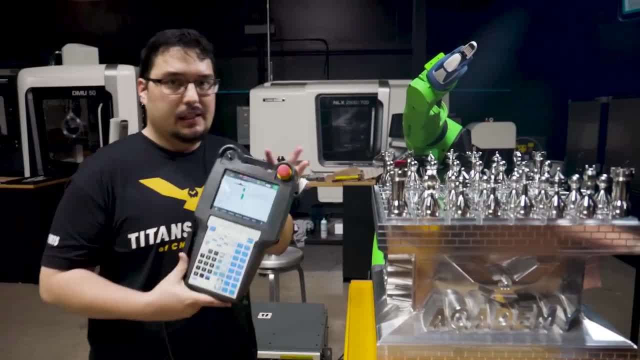 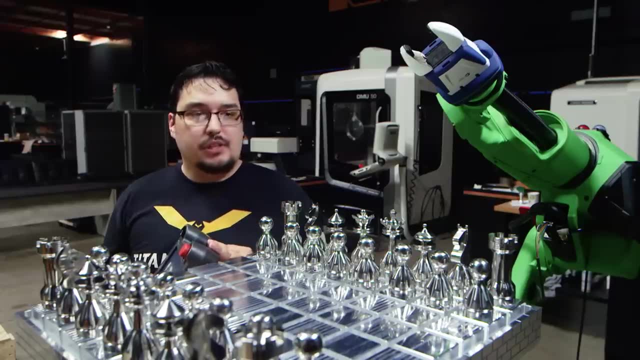 So we fired up the machine. I've got this guy here, which is the teach pendant, And this is basically the handheld controller for this robot. With the teach pendant, I can do everything from jogging the robot to programming it, to even controlling things like 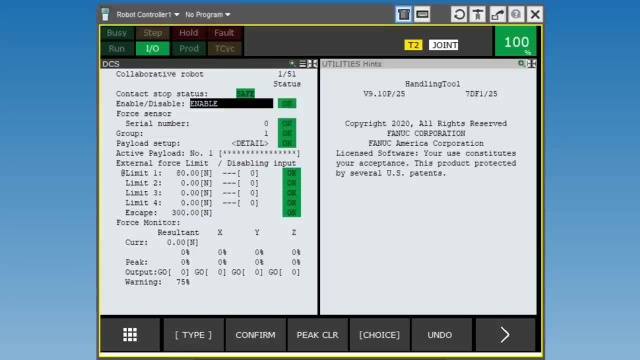 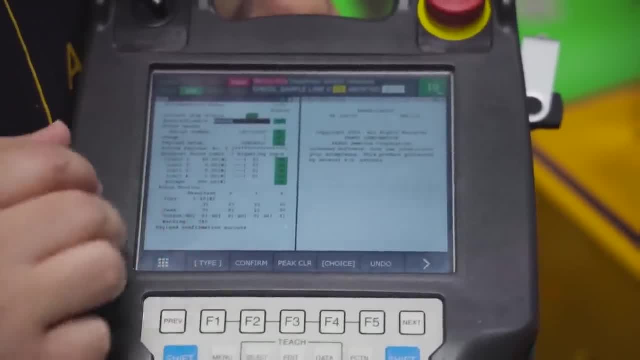 this claw here. This is the first screen that shows up when you start up the robot, So let me give you a quick rundown on the panel. The top screen is a touch screen. I have it set for two different windows so I can have my program on one screen. 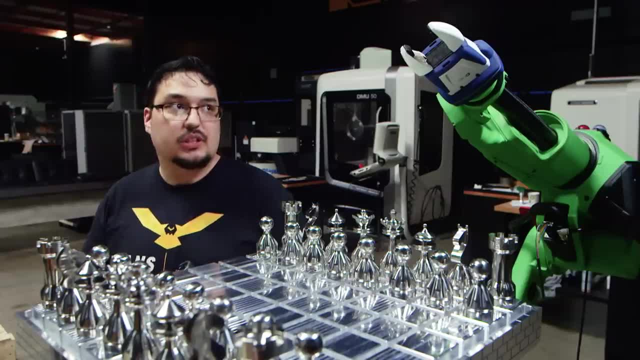 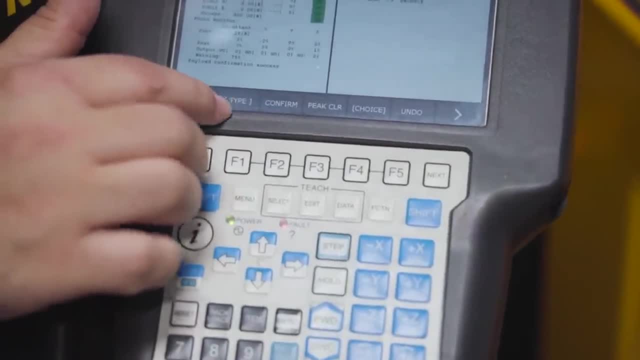 and I can have things like my position of my robot or the controls for the claw up. in the other You have these F keys which all correspond to these things here. These will change depending on which window you're in. Anything in blue here means that you need to hold down the shift key. 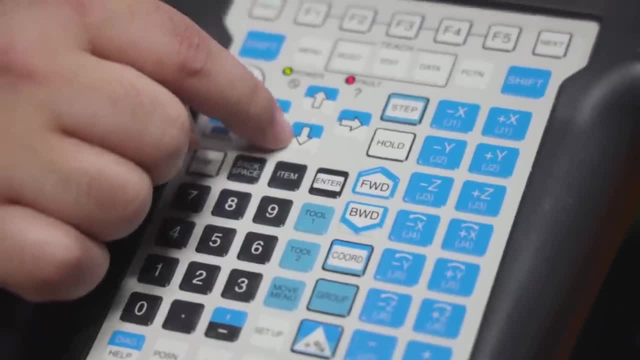 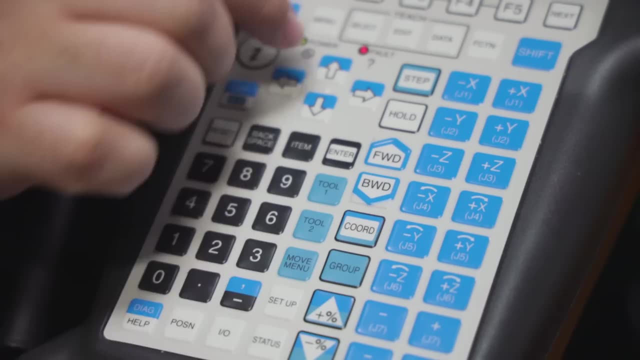 in order to run it. If it's in blue and white, that means it has an X key. If it's in white, it means that it has an extra function when you hold down the shift key. So all of these buttons on the side here, these are all to jog the robot. You have them. 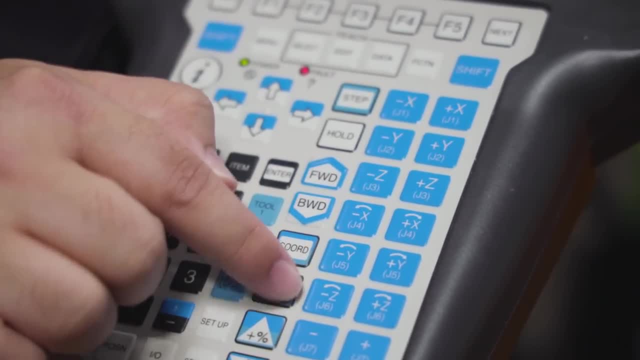 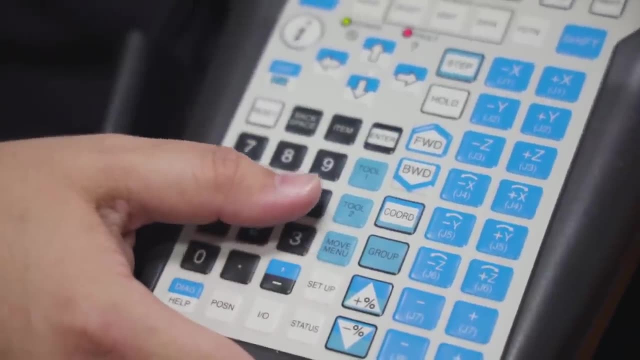 listed by axis, and you also have them each with their own joint number: Joint 1,, 2,, 3,, 4 and so on. So in order to jog the robot, you need to hold down the shift key and push one of the joint buttons and keep it held down. It kind of acts as a safety, so that 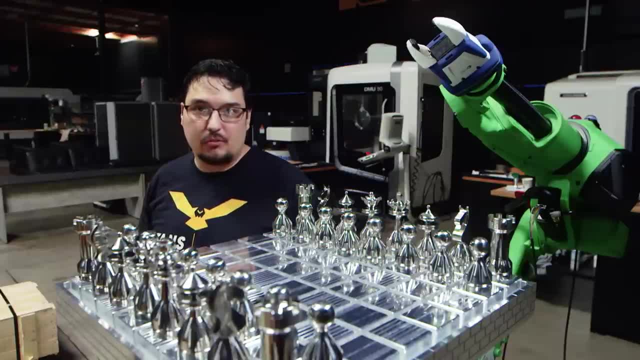 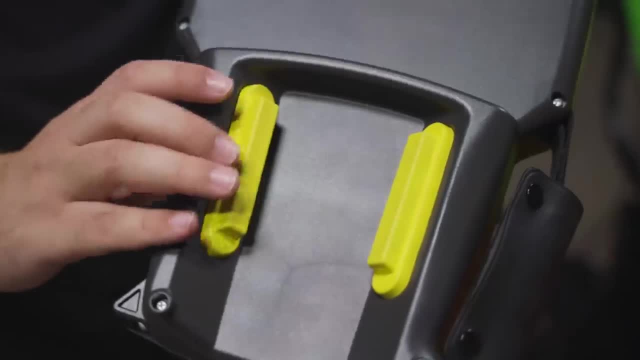 you need to constantly hold that down. That's only when you're programming the robot or when you're in teach mode, which i'll go over. two other important things to know. on the back you have these things here which are called dead man switches. you can push them in one. 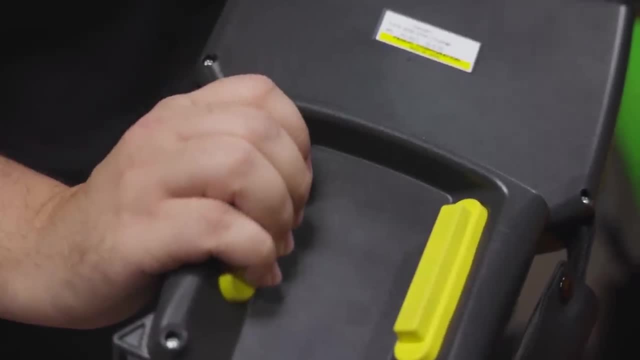 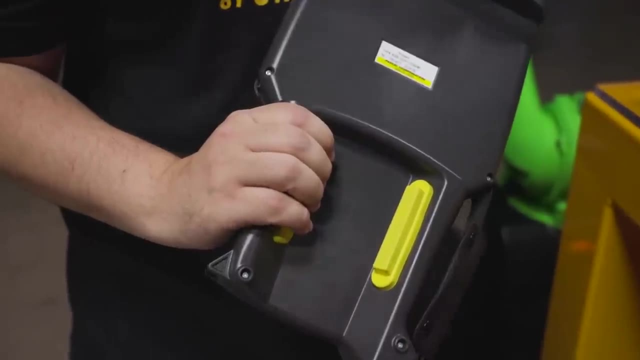 times very easy. and then the second time you kind of have to push in when you're using the teach panel and you're in teach mode. you need to constantly have this pushed into that first click in order to do anything with the teach panel. that's another safety feature. that's on. 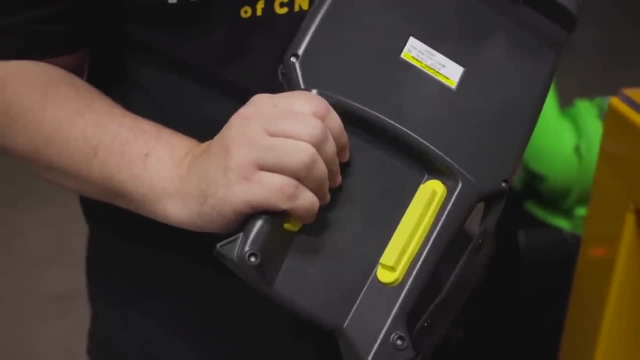 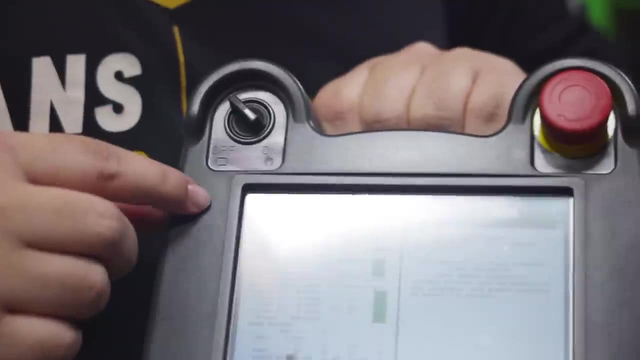 this robot. the second click when you push it all the way in. that acts as an emergency stop. the other important thing: at the top here you have an on and off switch here, that's to tell it if you're in teach mode or if you're in auto mode when your robot's all programmed and you're ready to run. 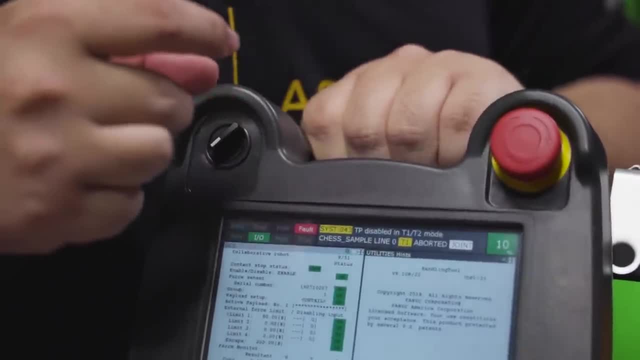 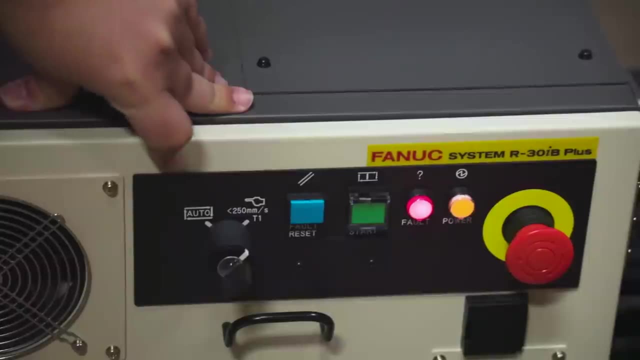 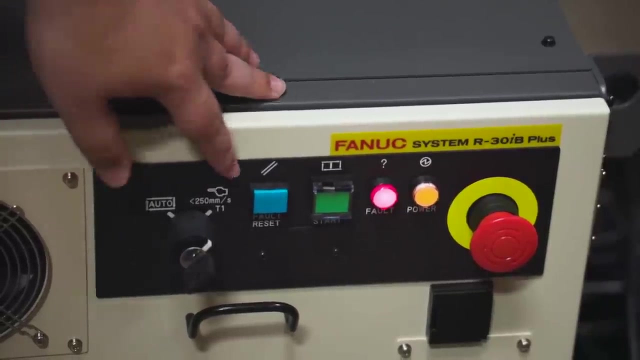 through your program. you need to switch it from teach mode to auto mode and from auto mode you can no longer use the teach panel. you have to start using the buttons on the robot controller. you can see the robot also has an auto mode setting and it has one that says t1, which is 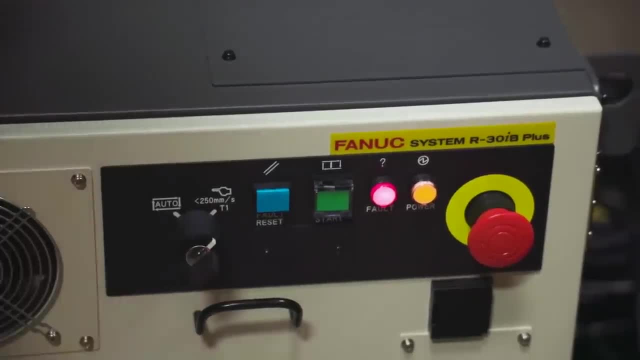 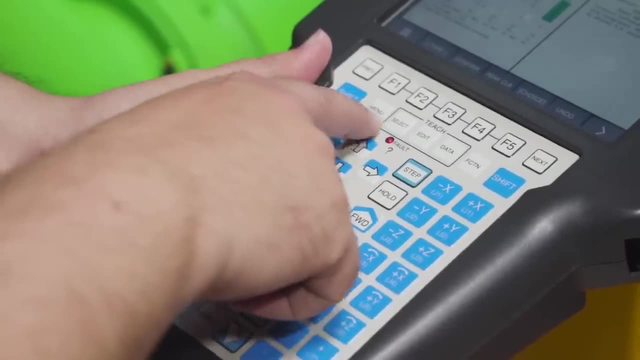 basically it's in teach mode here. so when we're ready to start running the robot, we're going to switch that to auto mode. the first thing i'm going to do is i'm going to make a new program. so i've got these teach buttons here. i'm going to hit select to bring me to my program menu from. 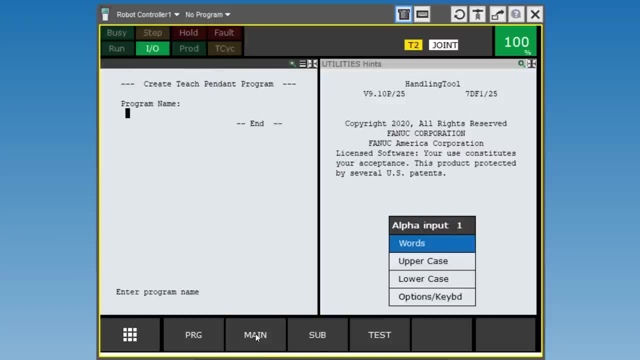 here i'm going to hit create. we're going to create a new program and now i'm going to enter a program name. so i'm just going to call this just2. now we have a blank program. let's start off by giving our robot our first move. so i'm going 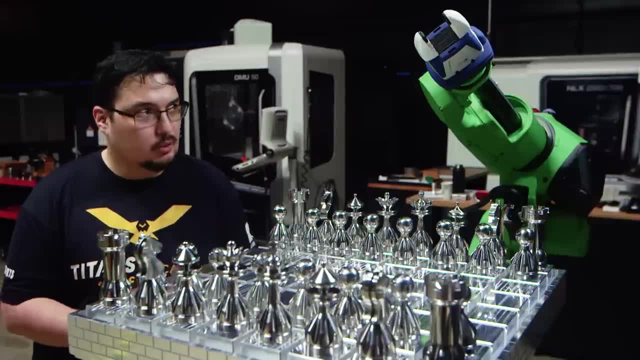 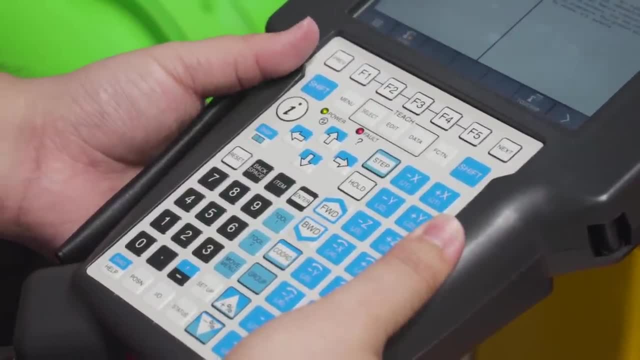 to start by giving it kind of a home position for the robot, its starting point: push on my deadman switch. i'm going to hit reset because whenever i let go of the dead man switch it gives out an alarm. i'm going to hold down shift and then i'm going to select which robot joints i want to jog. 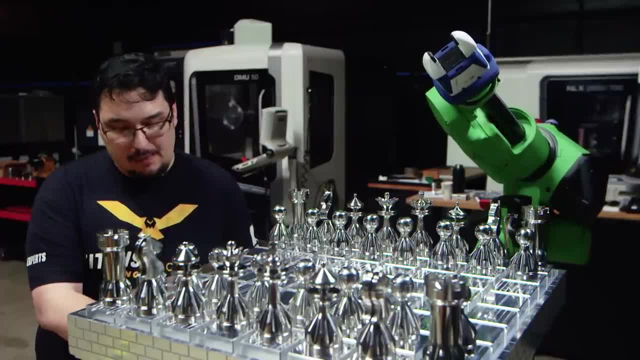 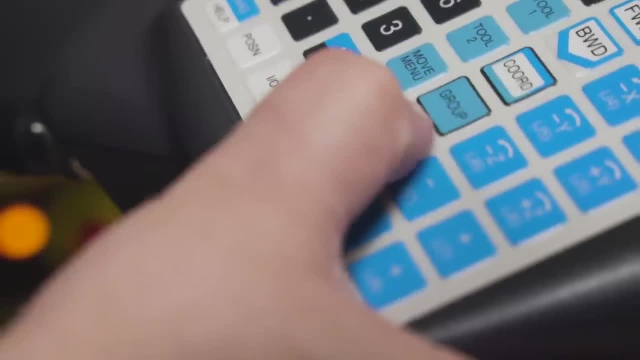 you can see it starts off a little bit slow. i have my rapid when i first turn on. the machine is set to 10, so you have these percentage buttons at the bottom of the panel which will increase the rapid on the robot. if i hold down, shift and hit one of those, it skips the percentage. so it goes. 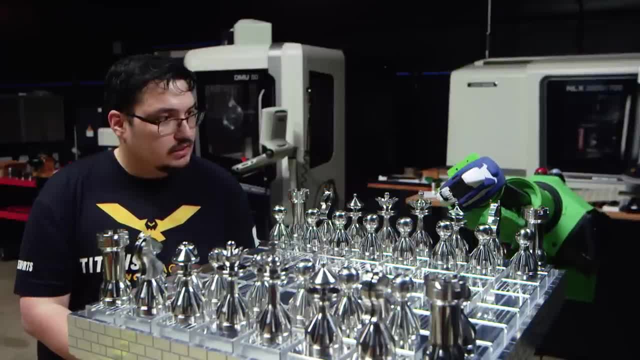 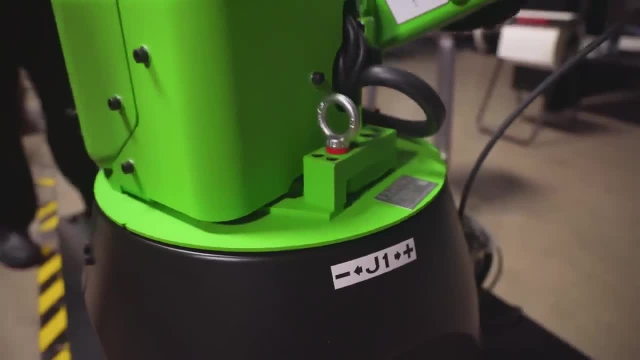 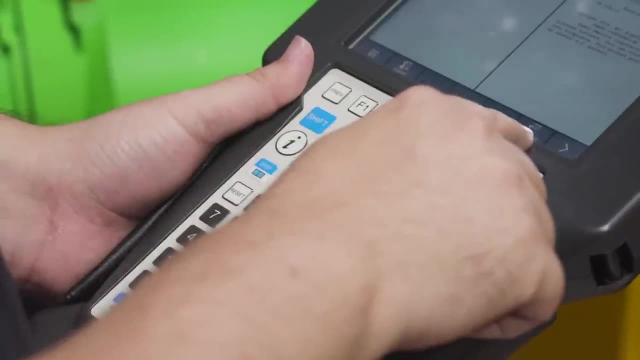 up to 50 and then 100, get the robot in kind of a nice starting position. once i've got my robot into a position i like- and i want that to be my first move- i've got these icons here at the bottom of the screen. you have point and you have touch up. so 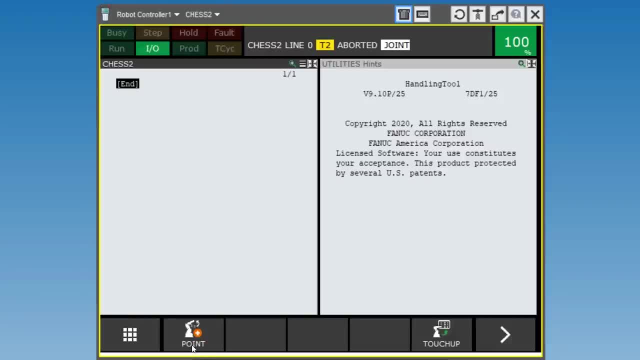 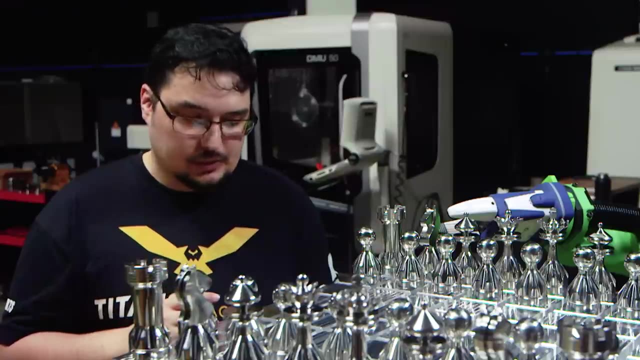 the one i want first is a point. it brings up these options here, which is what kind of motion i want this point to be. so you have fine motions and you have continuous motions. the fine motions will stop. every time it hits that position, it'll slow down and stop, and the continuous motions will. 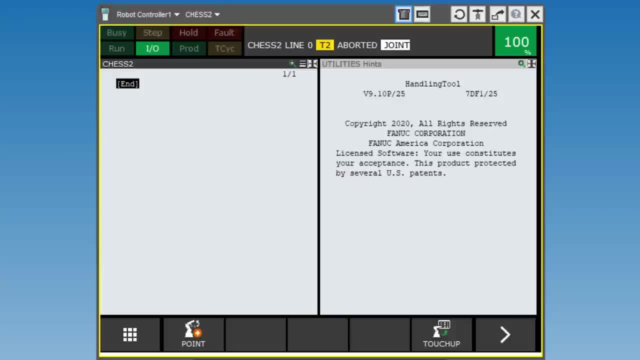 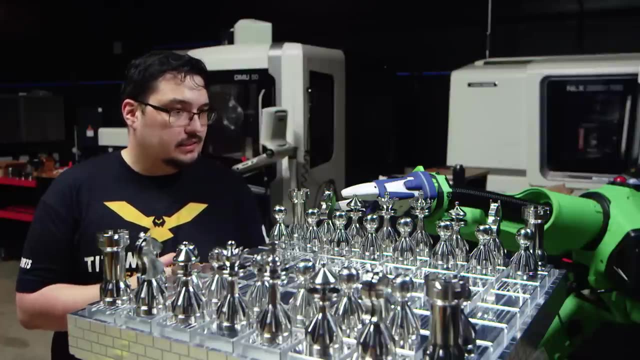 constantly move to make one fluid motion. for this tutorial we're just going to use fine motions. i'm going to hit 100 fine and hit enter and you can see in my program it recorded that move there. cool, we got our point. let's go to the next step. i'm going to move this robot in front of the piece. 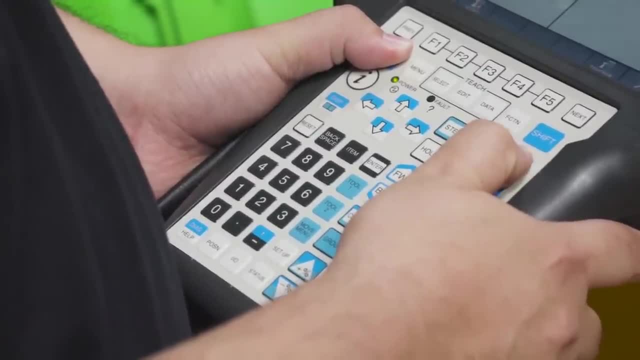 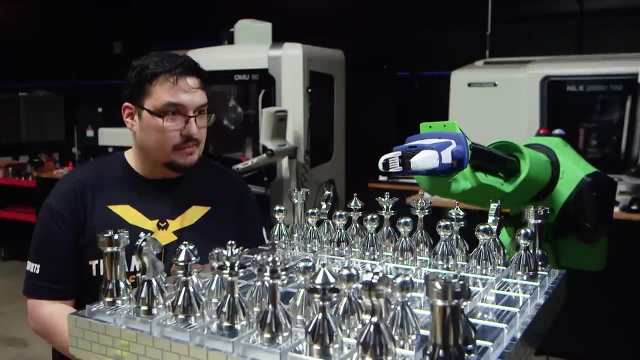 that i want to grab, so i'm going to rotate in the direction that i want to go. the piece that we're going to be grabbing is the queen on the board. i'm just going to move the joints until i find a point that i'm happy with. once i start getting close to the board, i'm going to drop my rapid down. 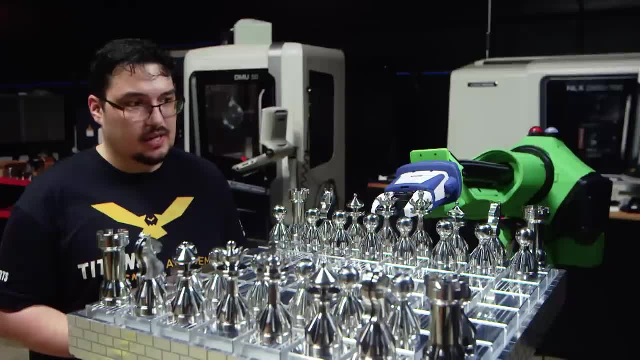 we're going to jog it into position to where it's close to a piece that i want to grab, but it's not quite all the way there. the reason is this robot's going to go straight from the first point that i selected. it's going to move straight to the second point, moving all its 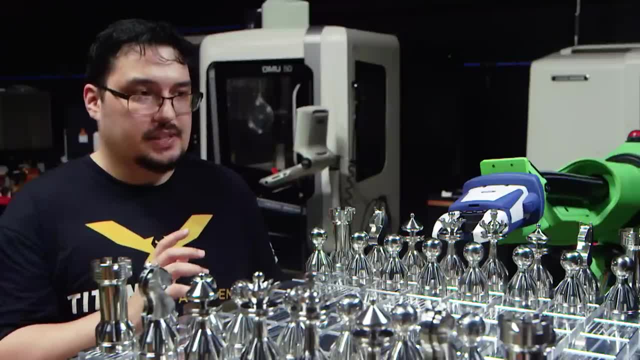 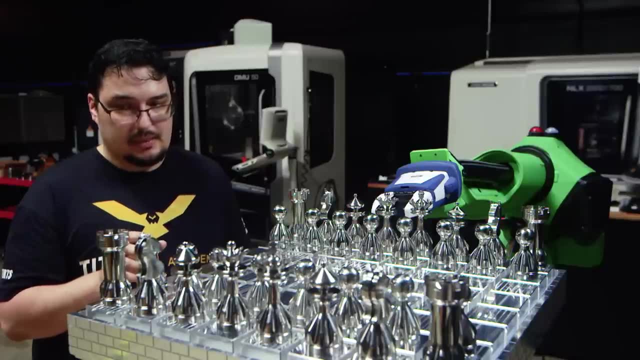 joints to get to its position. i don't want to go straight into the piece that it's going to be grabbing, because then it might knock over the piece or it might hit the board. i'm going to stop just a little bit away from what piece i want, in fact, just to be extra safe. 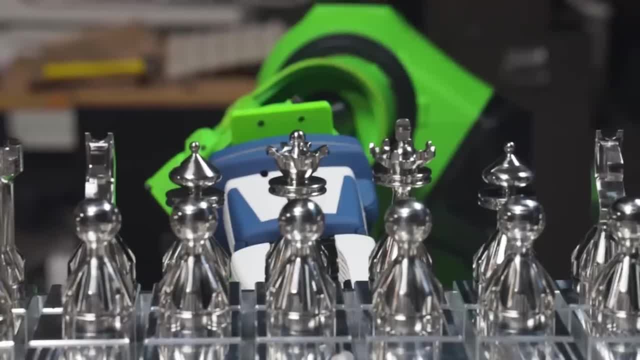 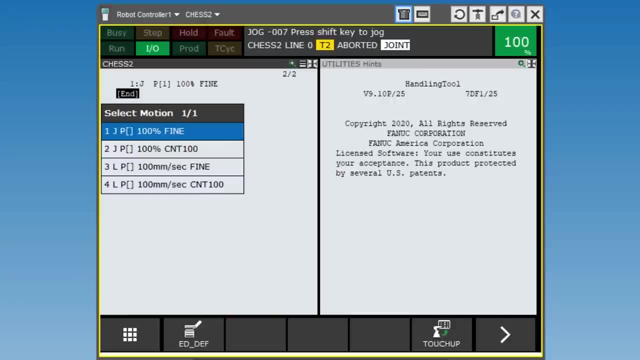 i'm going to back off joint two and we're going to make one more move where it's going to go to this position first and i'm going to record that point. so i'm going to do the same thing. i'm going to hit 100, fine, after selecting point and we recorded another point now from there. 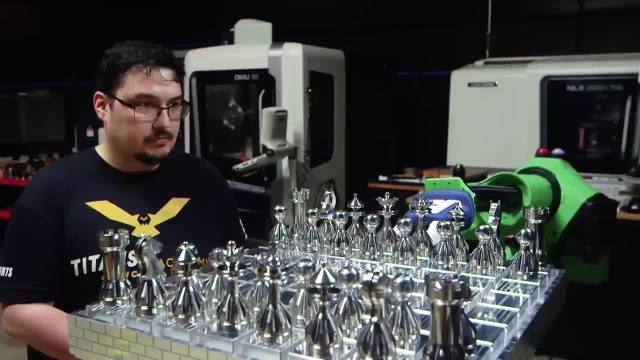 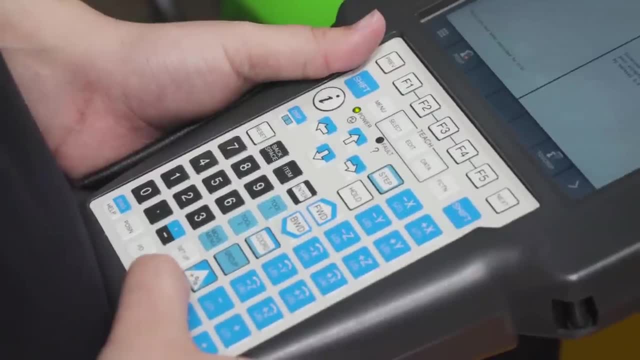 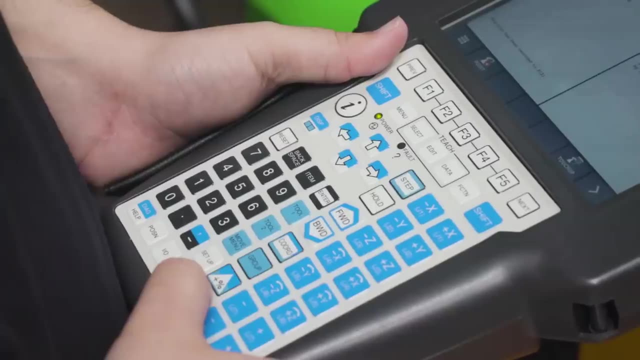 i'm going to go up joint two to where i was before. once. i'm happy with that. we're gonna add another point now here. i'm gonna get my claw around where i'm grabbing on the piece, so i'm gonna grab the top portion of the queen. let's drop my. 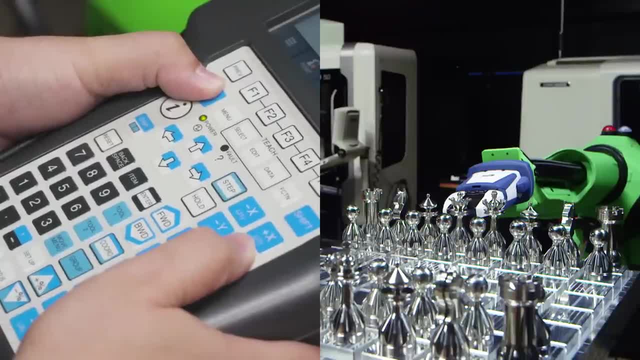 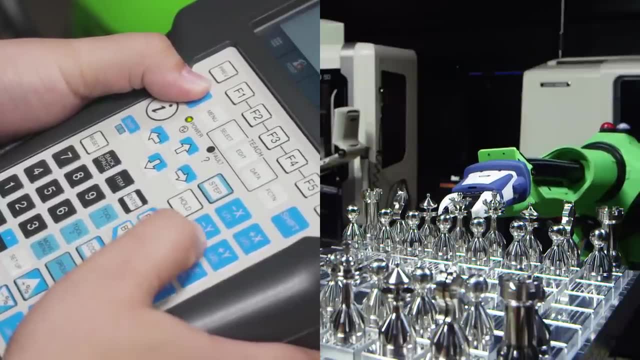 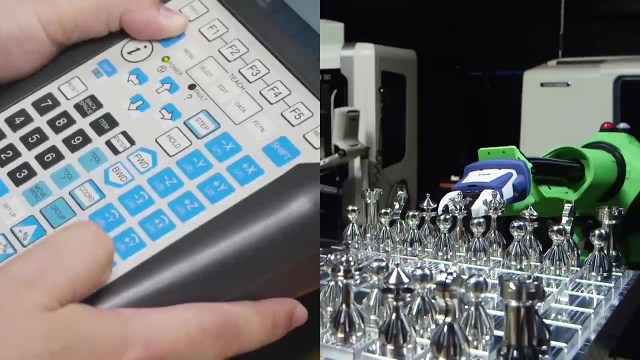 rapid down all the way to ten percent and i'm gonna be moving joint two and three until i reach about center of the piece and then i'm also going to rotate joint six- just a hair, because it looks like i could be centered a little bit better. 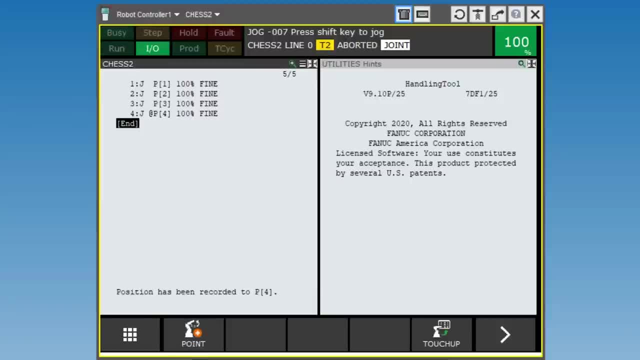 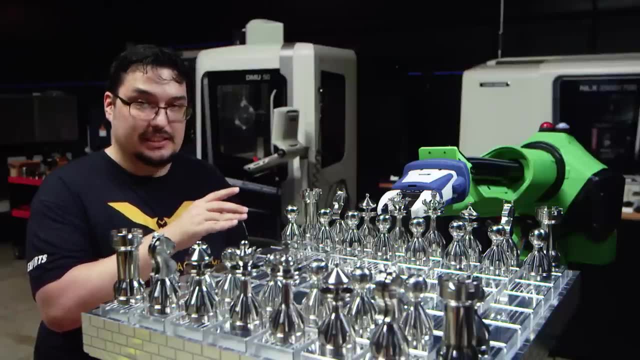 so if i'm happy with that, then i'm going to add that point. so now i'm ready to tell the claw to start gripping, i'm gonna actually grip the piece and then jog my robot with the piece attached to it so that i can make sure that when it's grabbing that piece there's no problems with. 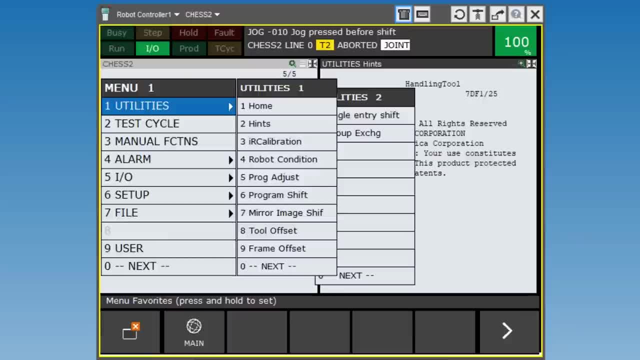 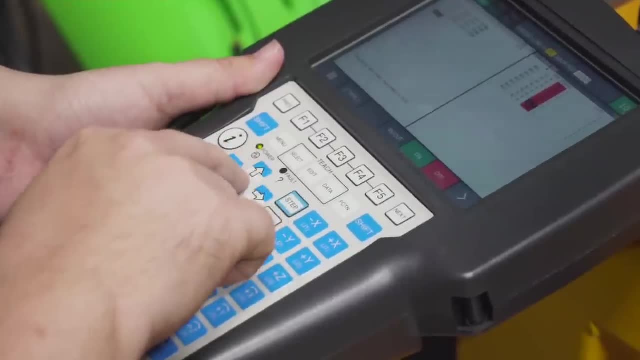 it moving it. i'm going to hit menu, we're going to go down to the fifth option here, which is i o, and then i'm going to go down to robot. these are basically switches on the robot, and for two of them the gripper is wired to it. so the last two here, seven and eight. 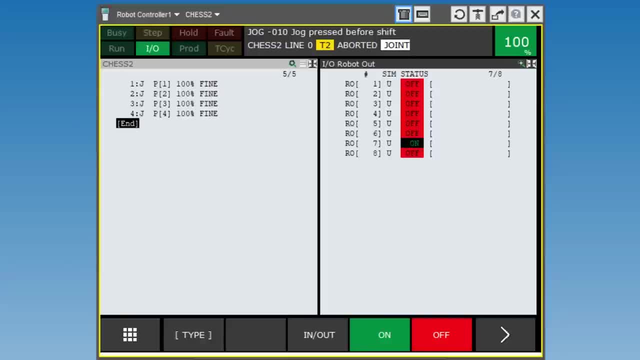 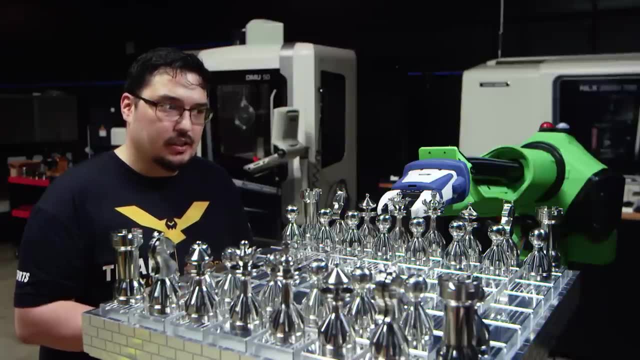 these are my claw controls. If I turn on seven, the gripper will close. If I turn that off and I give eight an on signal instead, the gripper will open. So one switch has to go off and the other switch has to turn on in order for the 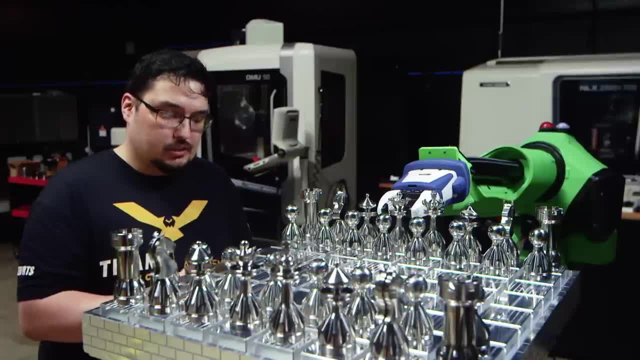 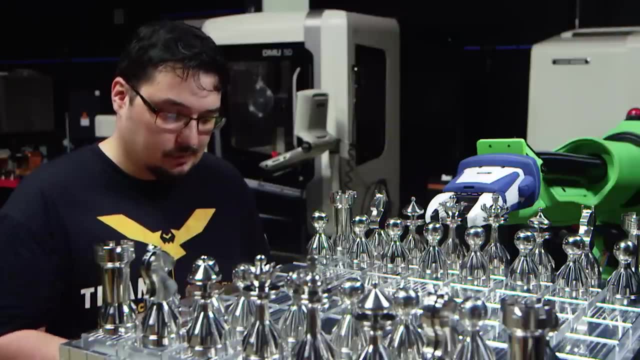 gripper to open and close. I'm gonna give these same commands to my program, so it'll do it automatically, but because I want to jog the robot with the piece attached, we're gonna use the gripper right now. So I'm gonna hit on on seven. 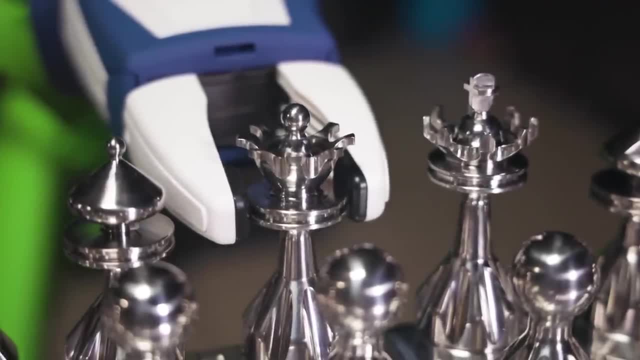 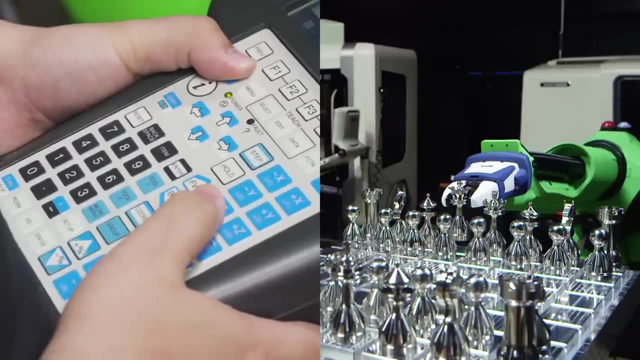 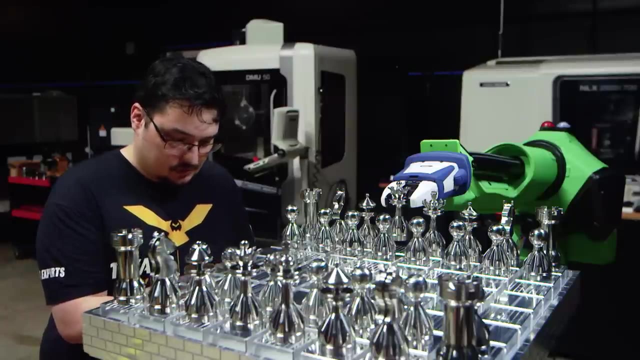 and that closed the gripper just now. So now, if I lift joint three up in positive, you can see it lifts up the piece. We're not going to record that move just yet, but let's go ahead and give my program those commands. And now, 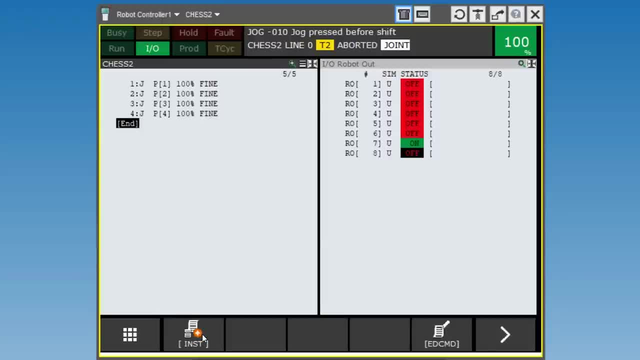 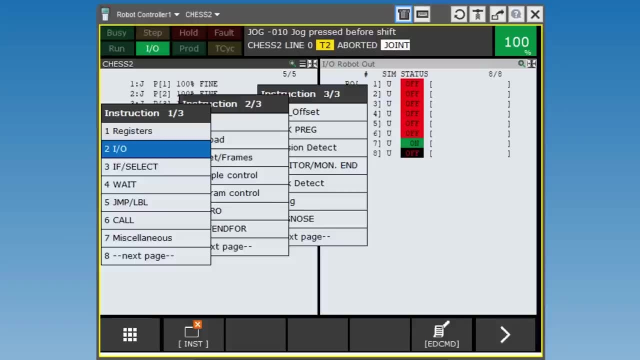 on these icons. I'm gonna hit this arrow over here. You can see. these are all the different kinds of instructions that you can give your robot. The one that we're going to be going over today we're gonna be using the I and O instructions. 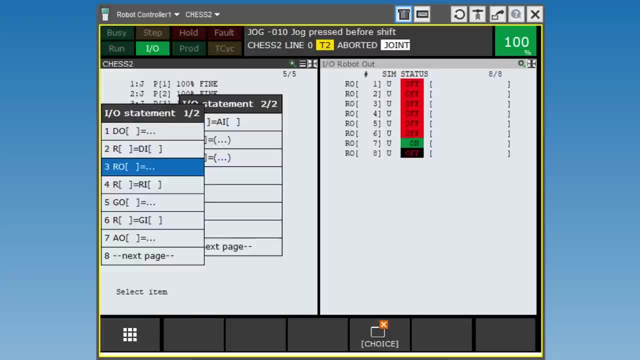 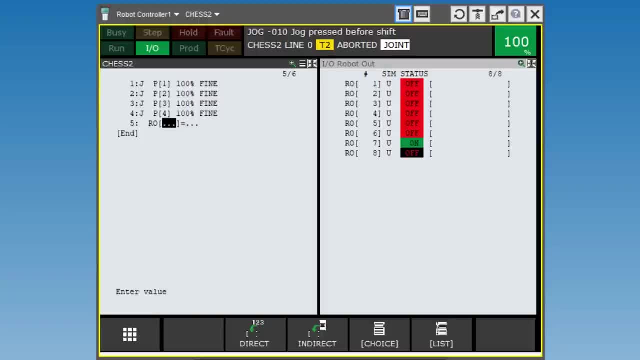 And now we have all these different statements we can give for this instruction. So we're gonna select RO, which is robot out. Now it's asking me to give a value for this R and O instruction, So I'm gonna tell it which switch first that I want to turn off. So I'm gonna change that to eight and then 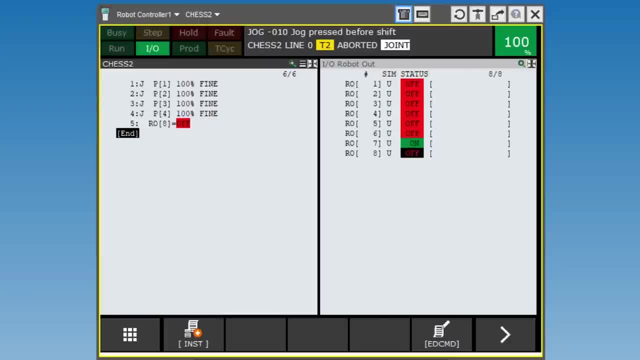 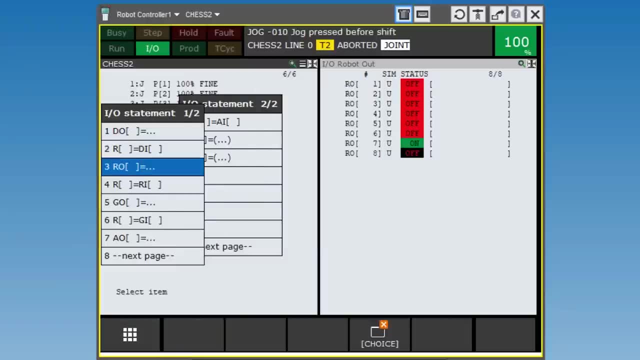 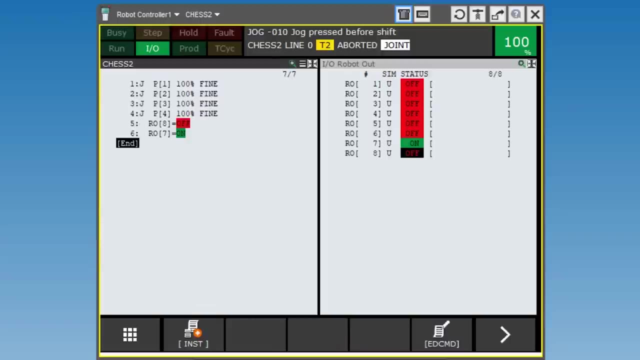 it's asking for an IO statement, So we're gonna turn that switch off. Now we're gonna add another instruction: INO RO. Now we're gonna turn switch seven, so we're gonna turn that on. So when it reaches that position, it'll turn off. 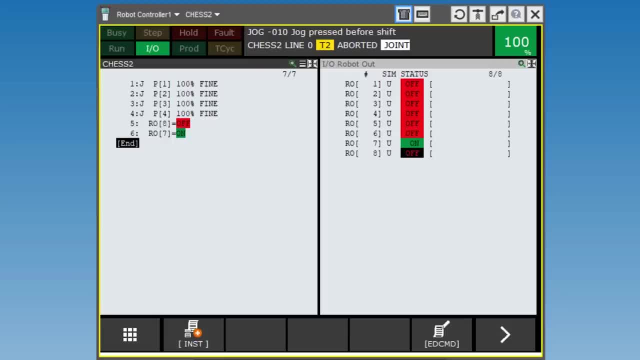 switch eight, turn on switch seven and then the gripper will close. One final thing before I make my next jog movement. after the gripper does its thing, I like to give it a little wait so that it has a second to actually grip the part. 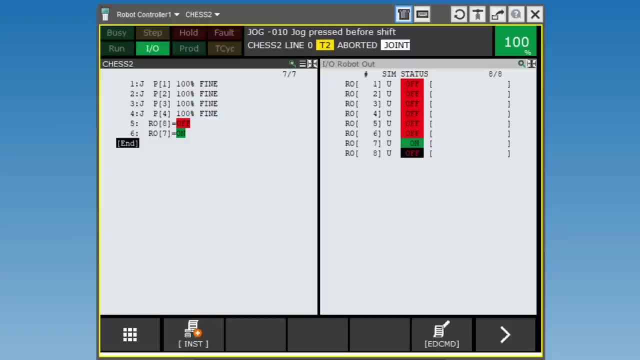 before it starts moving, because this happens almost instantly. So we're gonna give it another instruction and this time we're gonna select wait. You have all kinds of different statements here. We're just gonna go with seconds, so wait for seconds, And let's just say two seconds. That's what I did on the actual 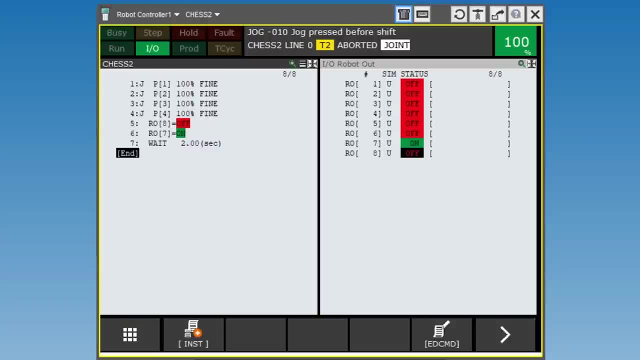 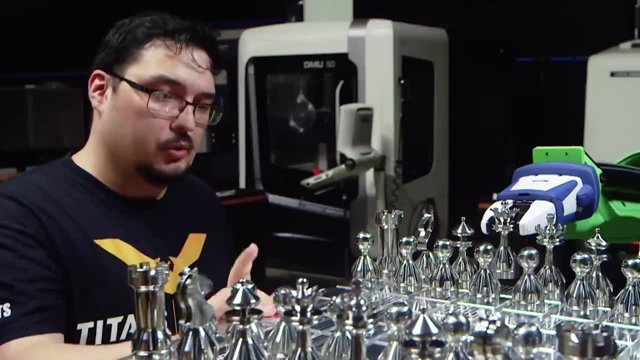 program. So after it does that grip it's gonna wait two seconds before it does the next move. So now that we're holding our piece, we're gonna lift it up. We can't just go straight to the section on the board that we want to go otherwise. 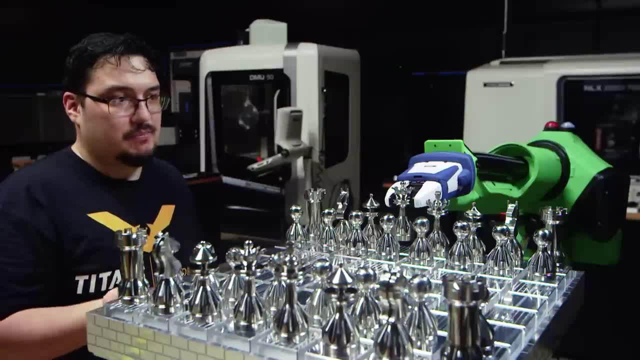 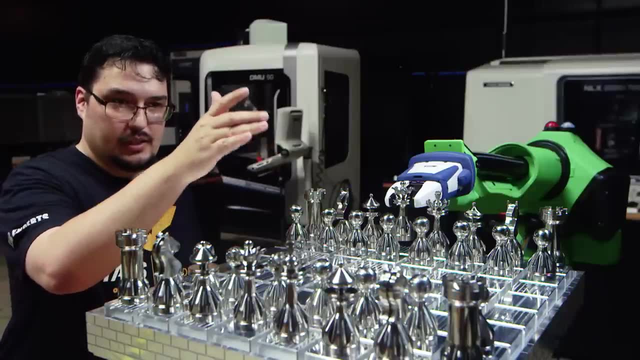 it's just going to knock all these pieces around. We have to lift the piece up first and get it up out of the way, and then we move it to around where we want to go, and then we're going to set it down. I lifted it up just now to show. 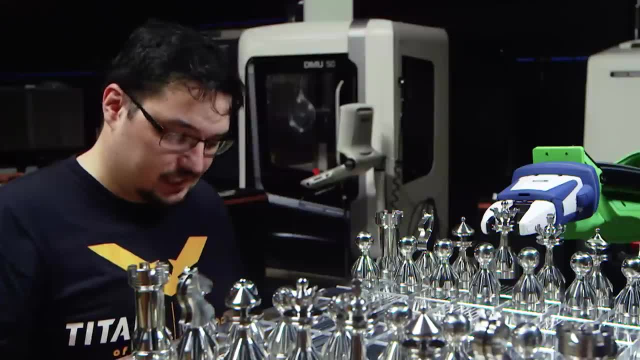 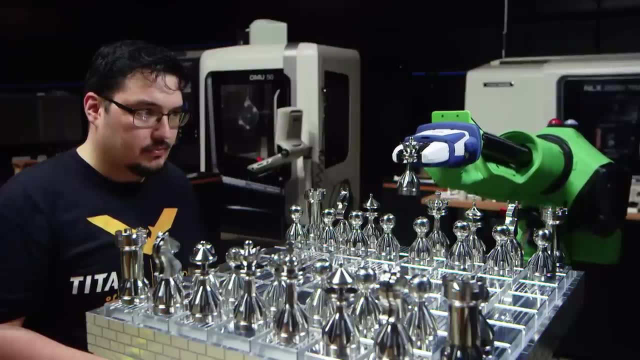 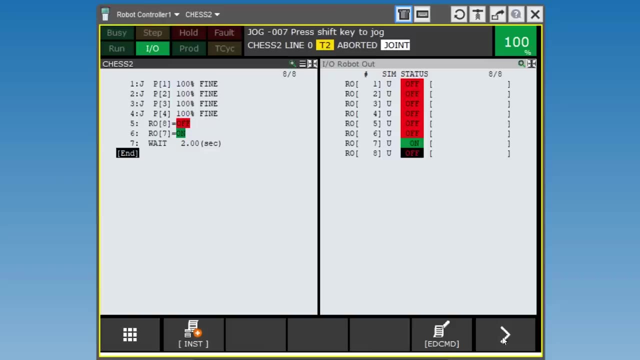 you the gripper and how that works. but I didn't record that point yet, So I'm going to lift it up just a little bit further before I record that point and get it to a position I like. Then I'm going to make sure my program window is. 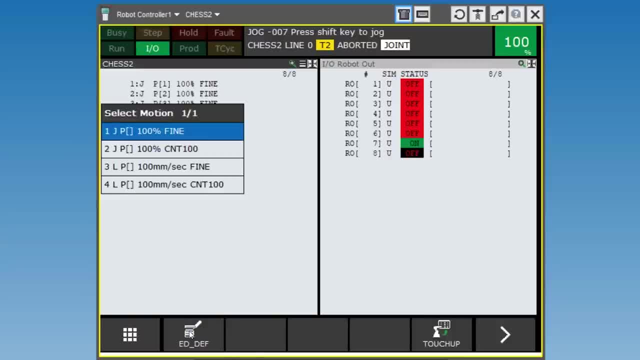 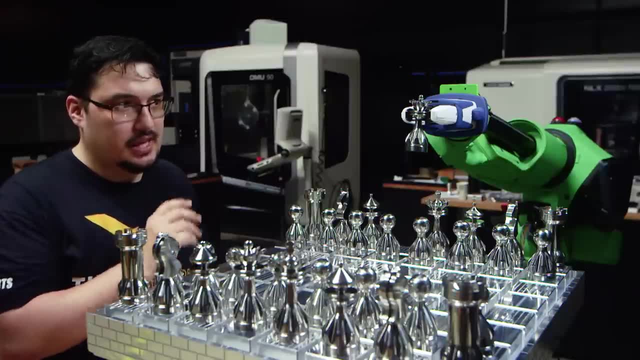 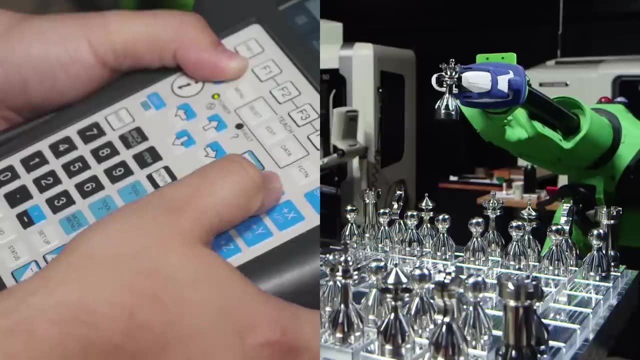 active, go down to the bottom and we're going to record that point right there. The robot's going to pick up the piece and go to that position. Now that I'm not going up against other pieces, I'm going to turn my rapid up. Let's move. joint two: 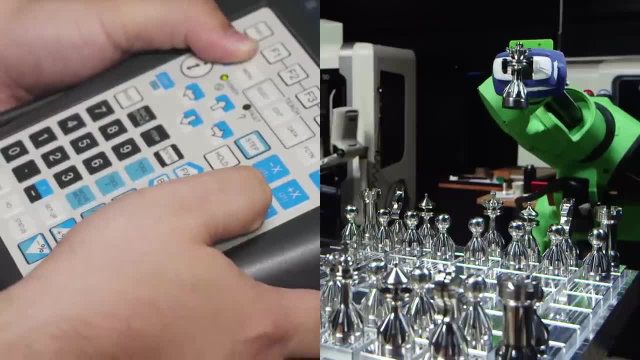 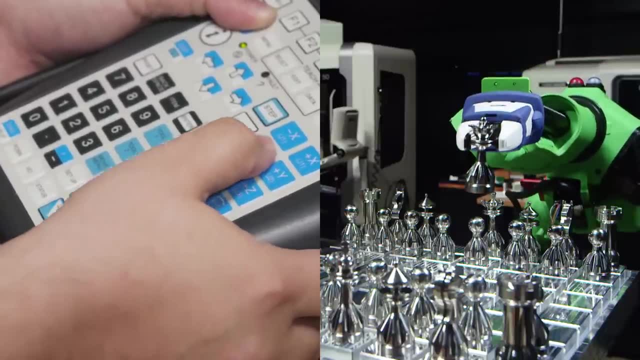 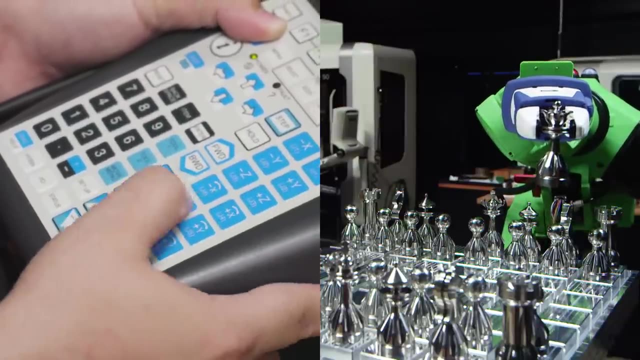 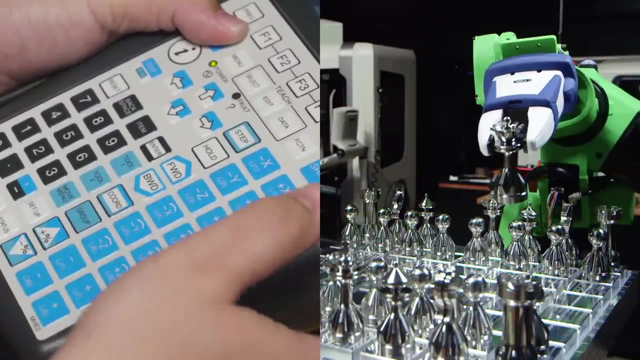 I'm going to move joint one and joint three, just a little bit. We're going to find a good position that I want to move this piece in. So you can see I'm moving multiple axes playing with different joints I've got. 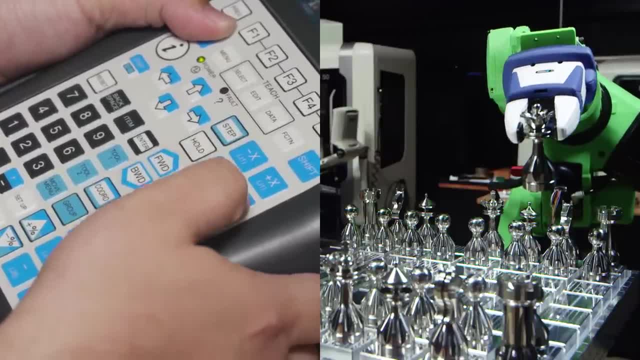 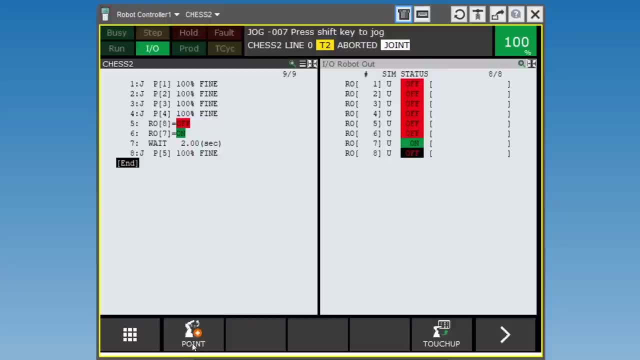 joint two here, joint three here, just trying to find a position that I like, close to that space that I want to move to. So this space right there. Once I'm happy with it, I'm going to click on point. I'm going to add that in. So now, 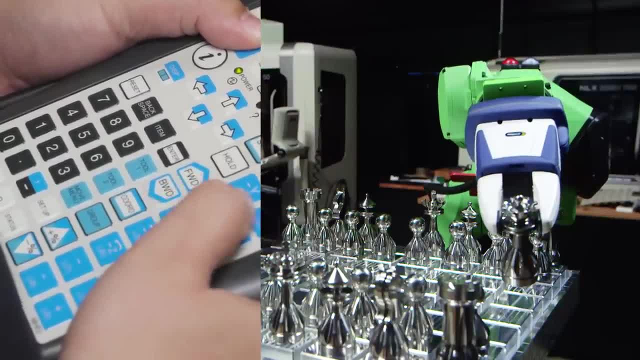 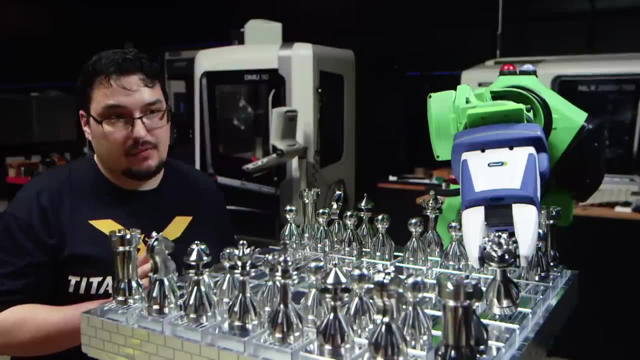 we're going to move it down so that it hits the space that I want, but I'm going to find a good angle to bring the robot. So I'm going to bring my robot right above the square that I want to use. I'm going to go down to the end of my program. I'm going to hit point. 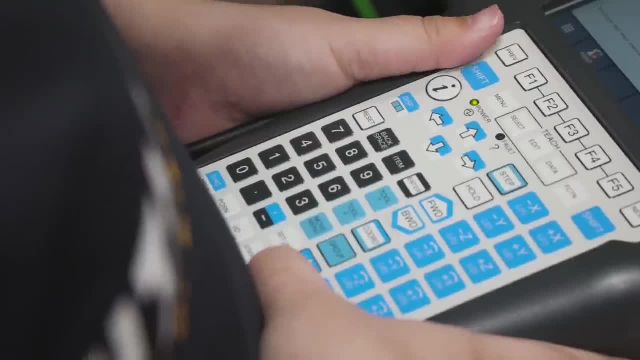 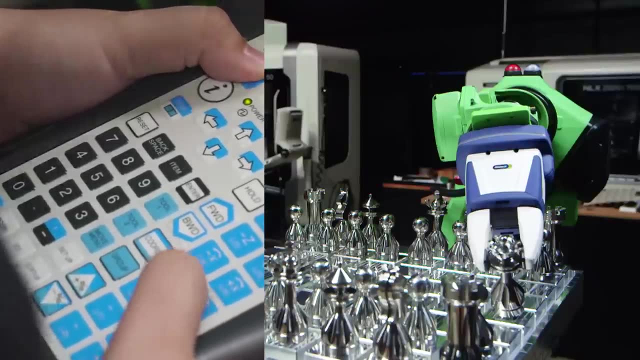 We're going to record another find move. So now I'm going to turn my rapid all the way down And we're just going to fine-tune this. I'm bringing down joint five to where it's just barely touching the table. So let's get the queen down So that when I let 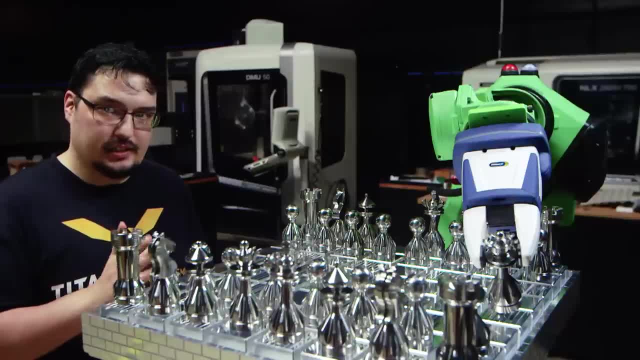 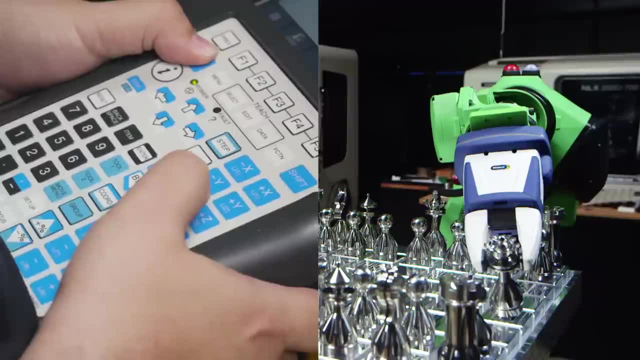 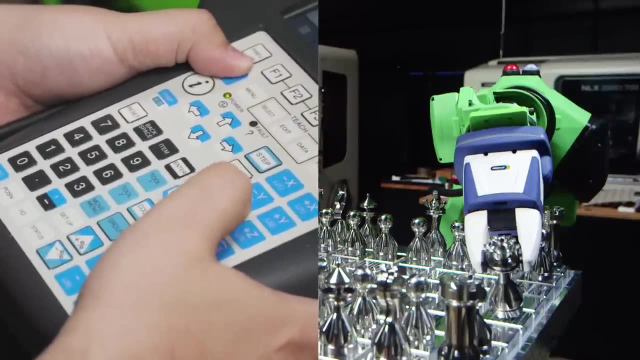 go of the gripper and it clamps, It's going to release the queen and it'll land on the space to drop my rapid all the way down. and then we're going to bring down joint 3 and move in joint 2, and i'm just going to go until i'm barely touching the table. 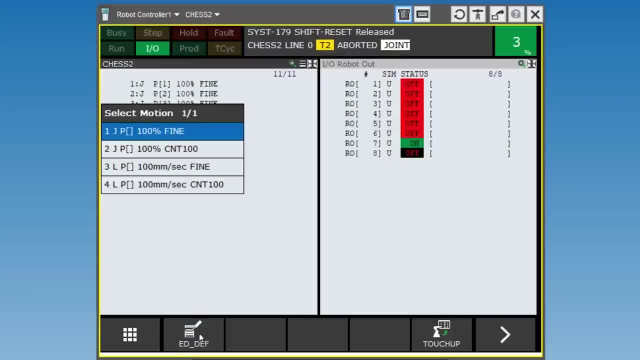 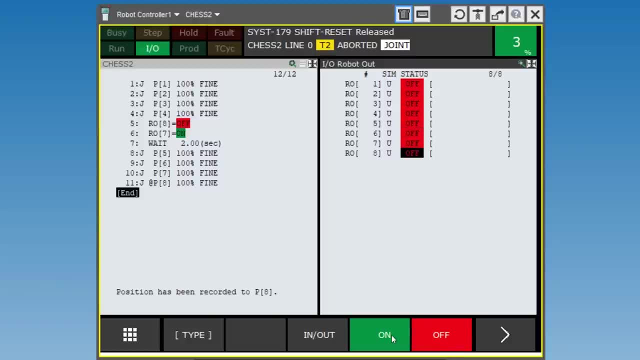 so get it to where i like it. we're going to record the point. so i'm going to go down to switch 7, i'm going to turn that off, and then i'm going to hit switch 8 and i'm going to turn that on. i'm going to give those commands in my program now. so we're going. 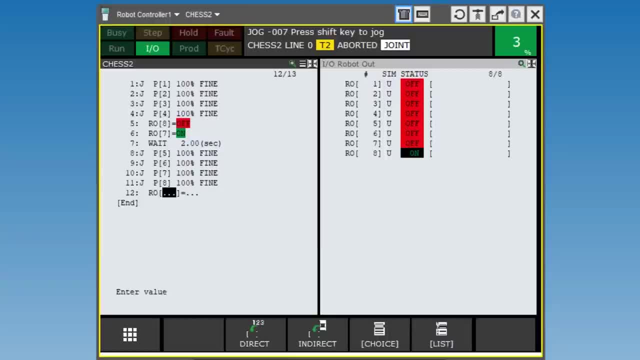 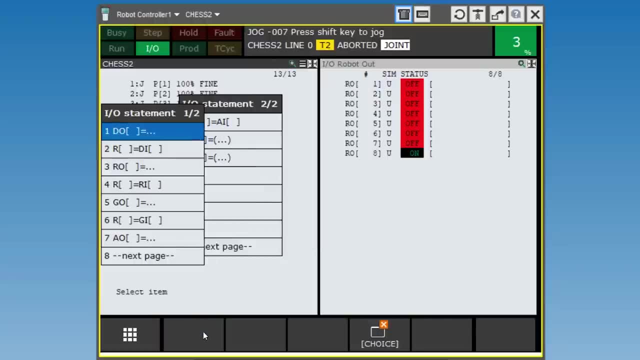 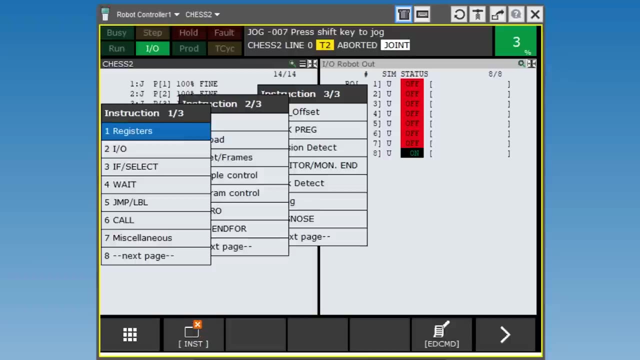 to go down to instruction io. then we're going to go to ro and this time i'm going to turn switch 7 off. so switch 7, turn off, and then we'll go do the same thing to switch 8, but that one we're going to turn on, and then, once again, we're going to wait two seconds, just like when we gripped on. 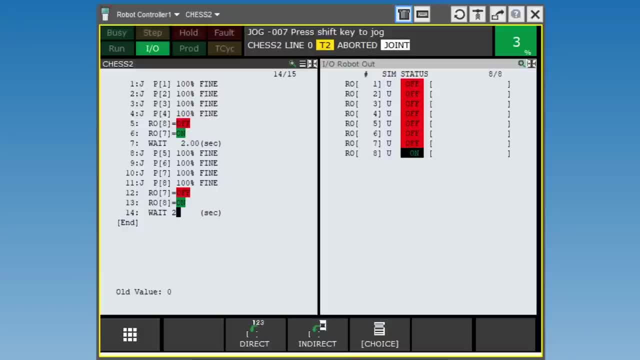 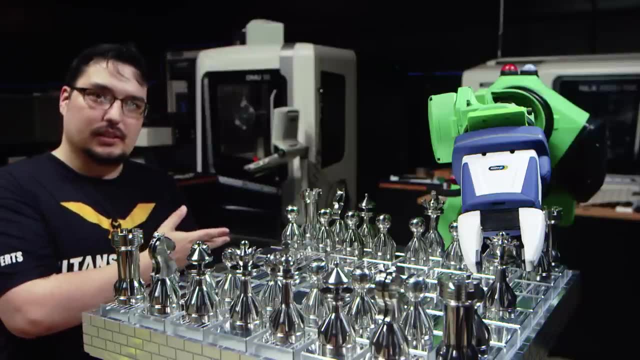 to the piece. so just think of all the different kinds of things you could have this robot do using a similar kind of motion. you can have it pick up all kinds of pieces, load pieces into a lathe- the possibilities are almost endless. once i'm happy with where it's at, we're going to move the robot out of the way. 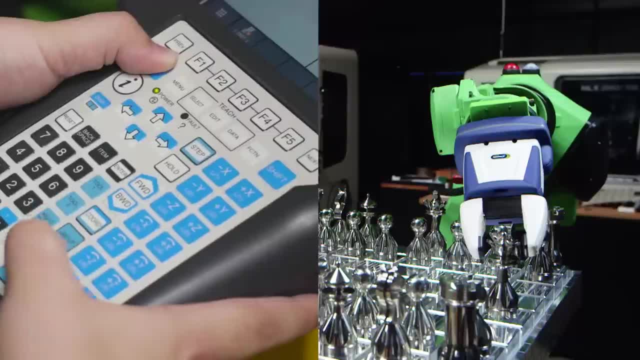 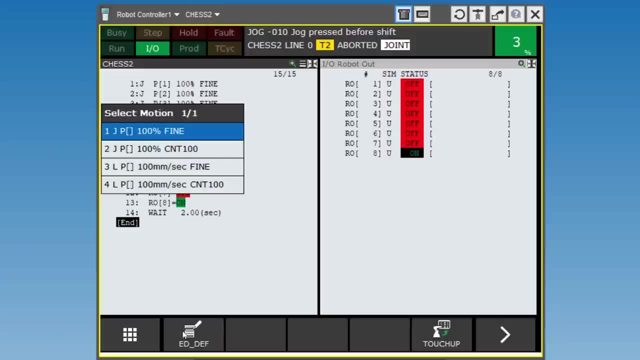 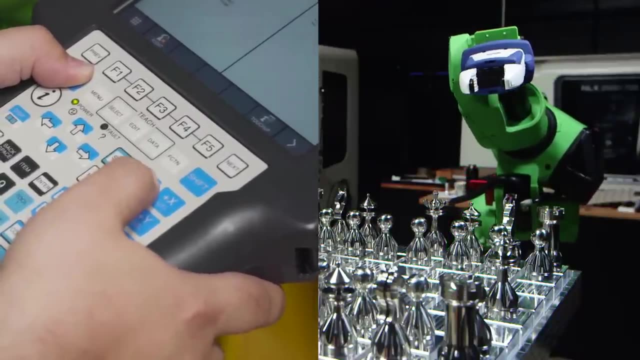 now. so i'm going to pick up joint 3, pick up my rapid joint 3: positive, let's just get it out of the way somewhere there. we're going to record that point. and now we're going to bring joint 2 all the way back. we're going to go joint 1. 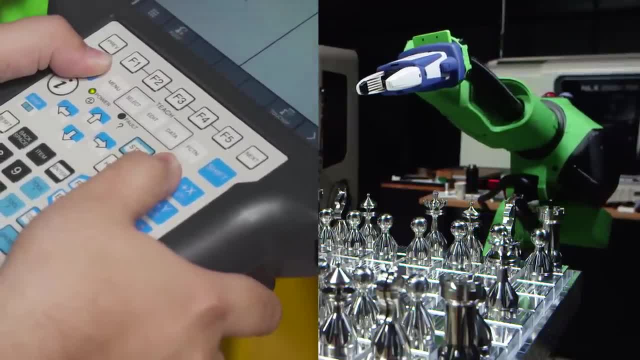 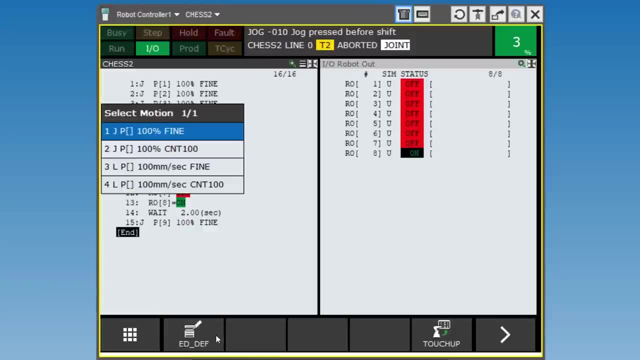 kind of move all the joints slightly. so i'm going to get it to this position here, add another point. the last move i'm going to do is we're going to bring it back to that first position i had. so now i'm just going to add another point, the same point where i'm at. 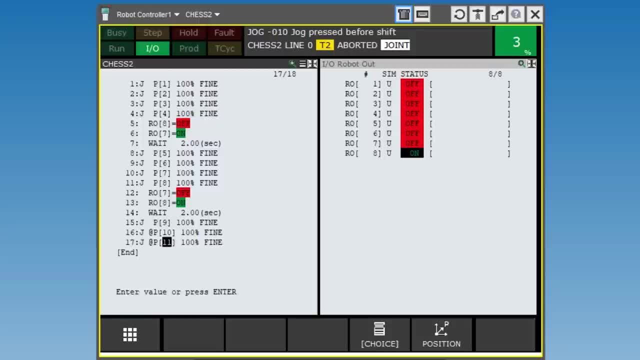 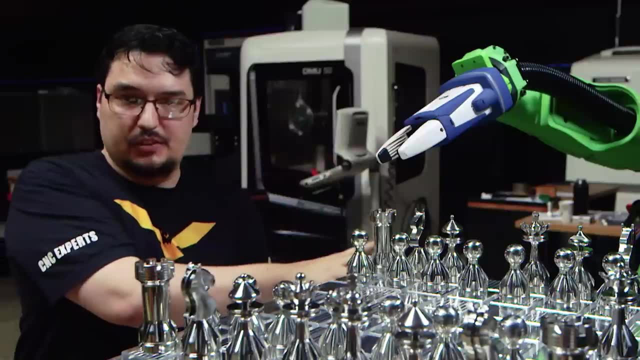 it shows up as point 11. but i'm going to change that point right now and i'm going to give it a value and we're going to say point number one. so from this point here it's just going to go back to the very first position that i had it at if i hold shift and 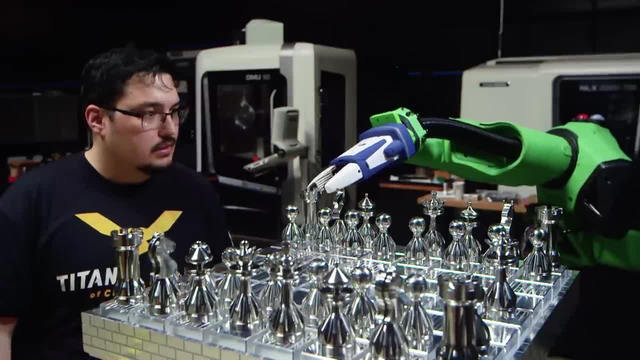 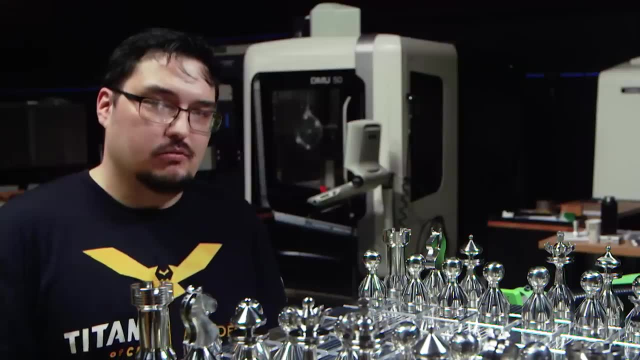 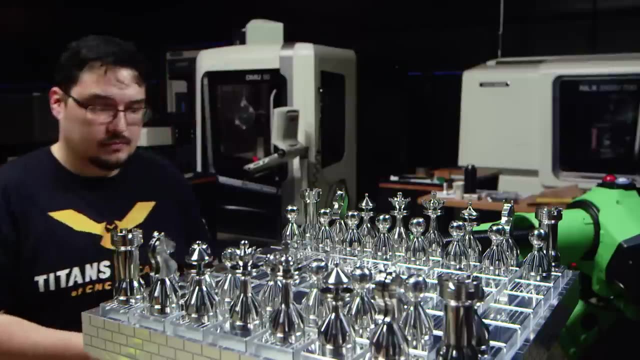 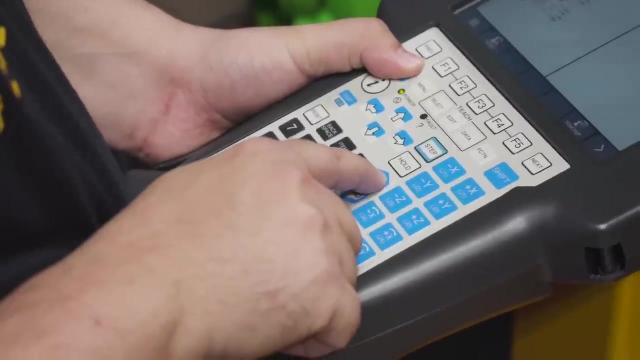 press forward. you can see it's going to go back and it moves to our starting position. we're going to run through it real quick, so i'm going to move my piece back and we're just going to step through or single block through the program and i'm going to hold down the shift key and we're going to push. 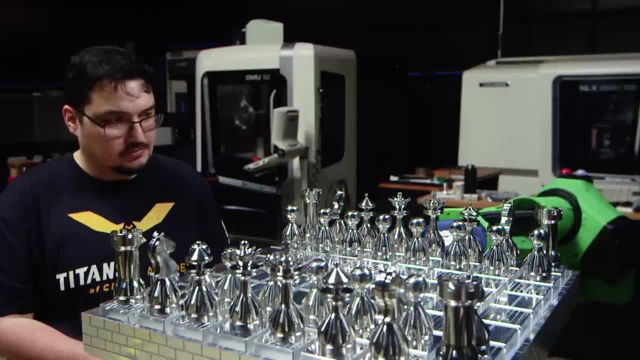 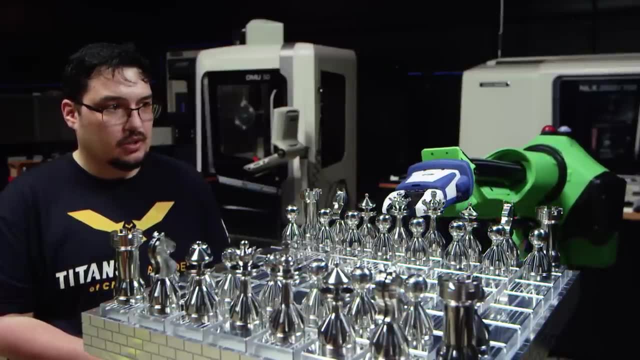 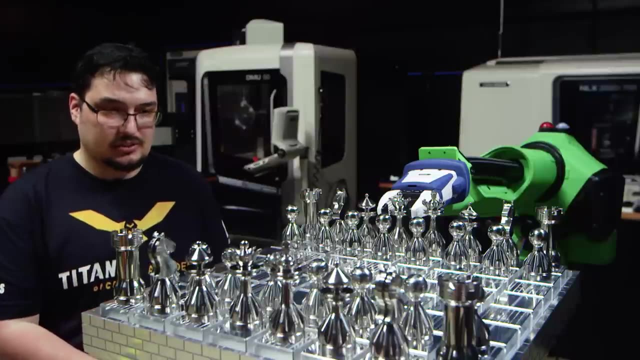 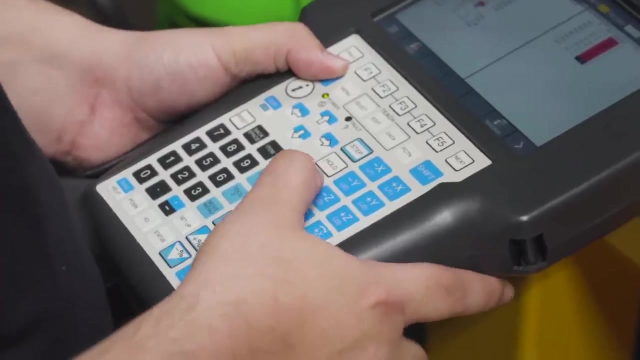 forward, so it goes to line two and then it goes to line three and you can see it's just going to go through all the motions now. so every time i push forward because it's on step mode, it stops. this panel also buzzes every time that it stops to let me know that it's ready for the next command. essentially, right now i'm proving. 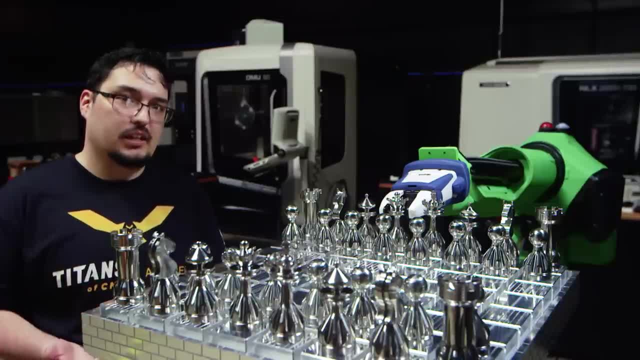 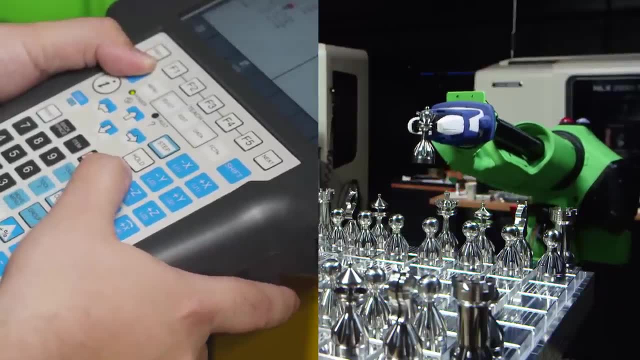 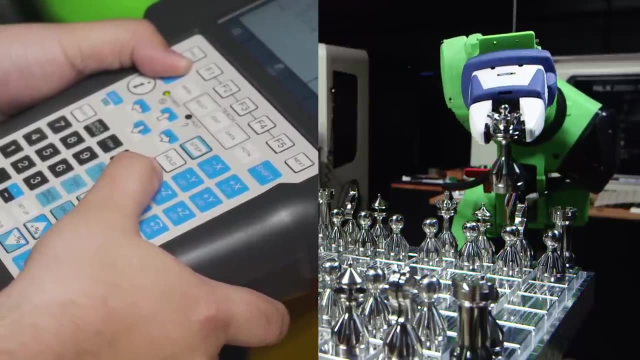 my program out. like i mentioned before, it's like a single block on a machine going through line by line on a cnc, making sure your program is good, it's going through, it went through our weight command, it's picking up the piece, going forward, bringing it down close. 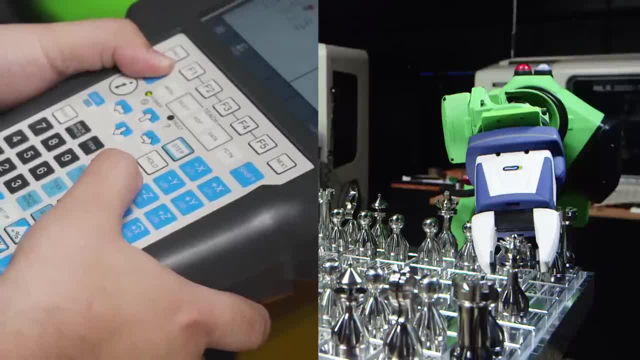 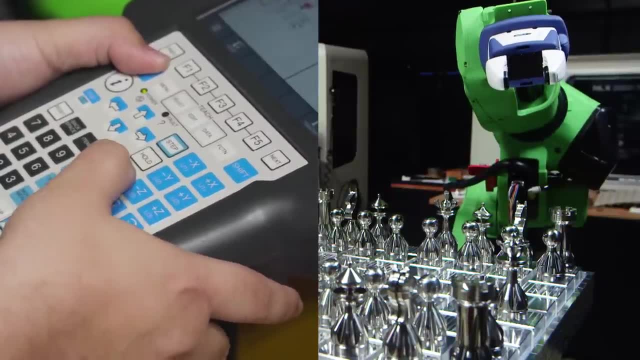 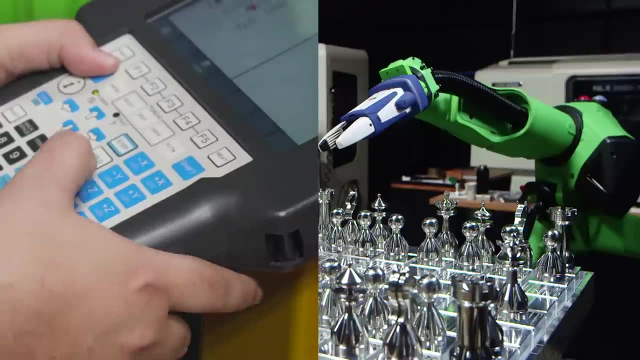 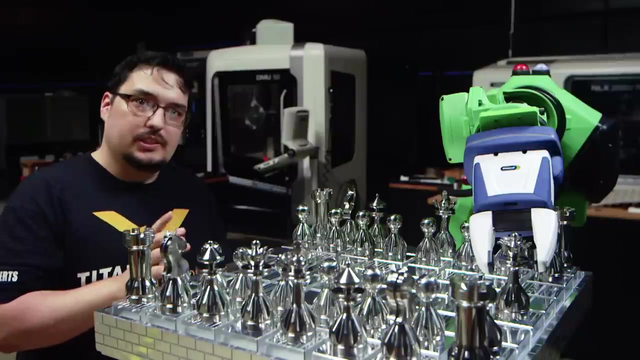 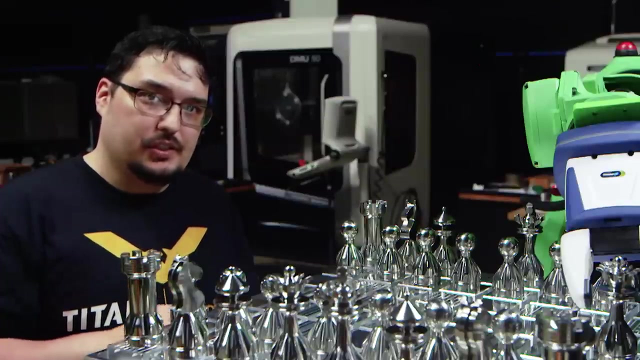 setting it down, it's waiting, comes back up and then goes into position. you probably saw that nudge when it lifted up from this point here. it moved the piece just a hair. it's really easy to fix up points if you don't like a line or you want. 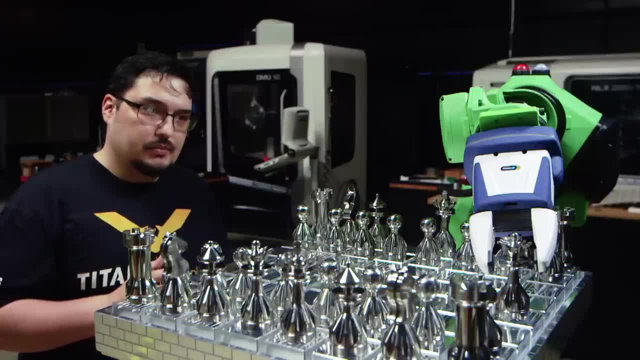 to change it to a different position. so all you have to do is switch it up a little bit and then from the position that you want to change. this is probably because i moved joint two a little bit too much in one direction because, like i said, when it moves to another position, it moves it. 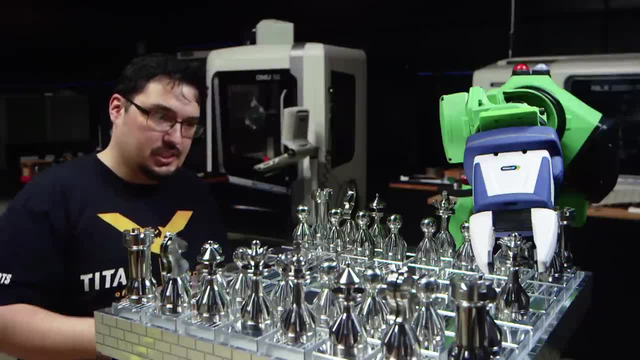 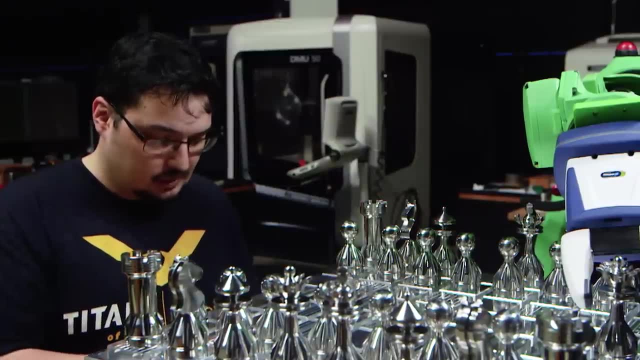 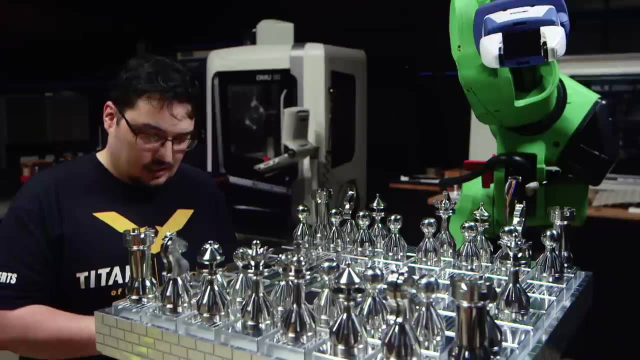 all at once. so it touched the piece just a little bit. so i'm going to shift up from here. this is that position from right after it lets go. this is point number nine on my program. i'm just going to move joint three up from this position- i'm going to make sure i'm on the line- and position one from: 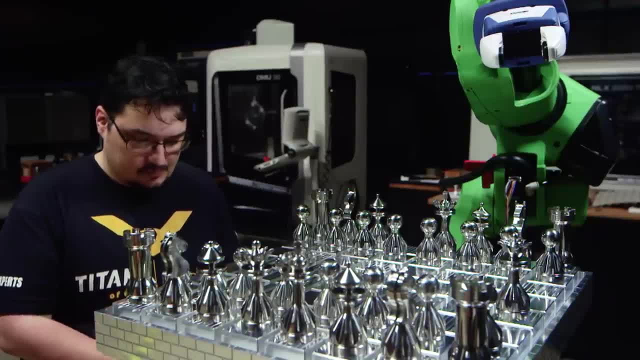 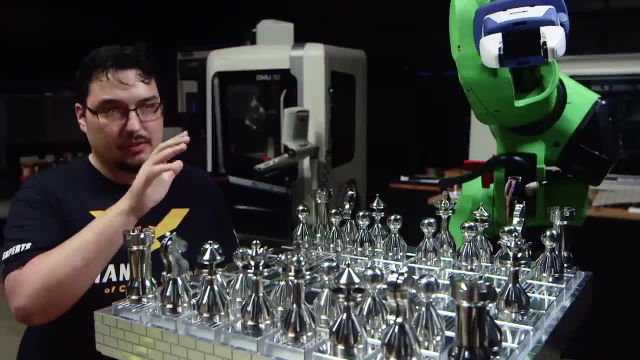 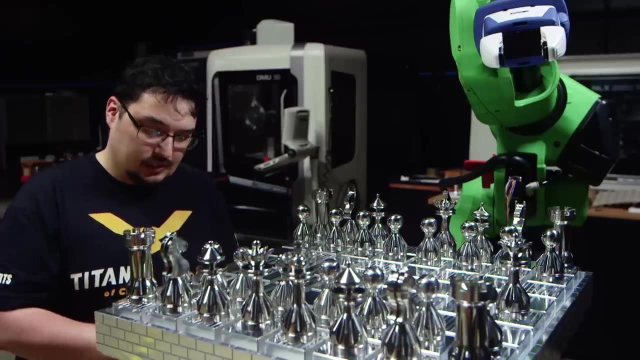 on the line that I want to change. so point number nine: I have touch up here on the screen so I can actually touch up that position and change it to where I'm at currently. so if I click on touch up it says press shift key. to record, we're going to hold down the shift key and hit touch up and then 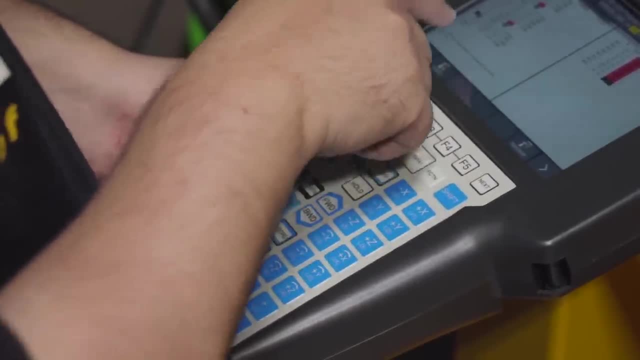 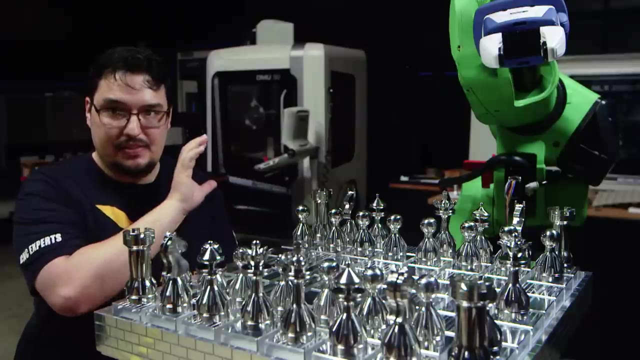 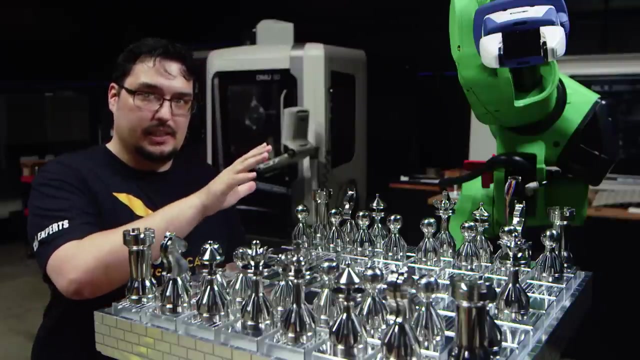 it says: point has been recorded to point nine. you can also see there's an at sign on my program. that means the position of the robot is at that point. it's very sensitive to collisions and impacts. if a piece is moving too much it might alarm out because of it. so it's very easy to 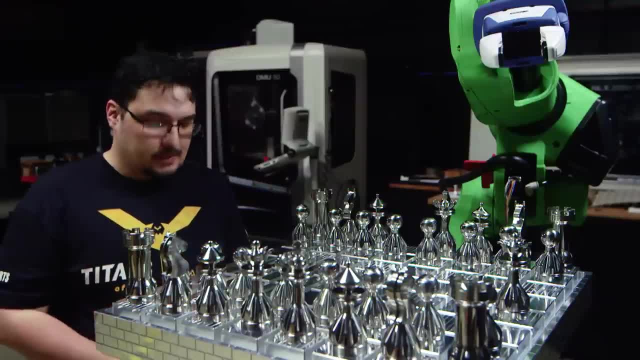 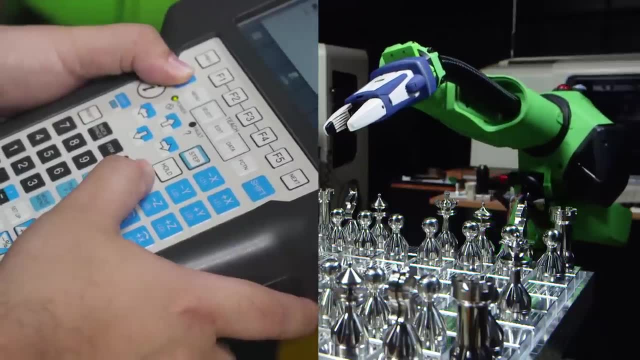 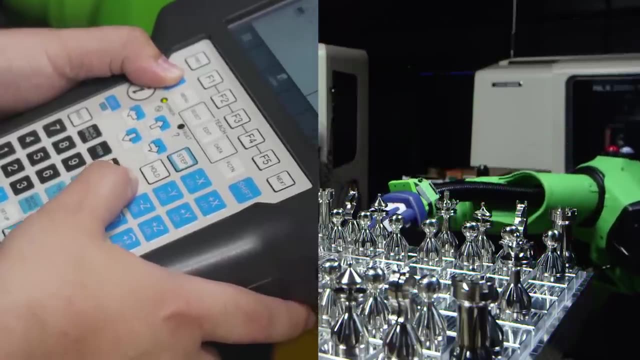 program and catch mistakes with this robot. so from our new point I'm just going to continue our program and you can see now it has no problem and gets back to our home position. So with that I think we're ready to run the actual program now. 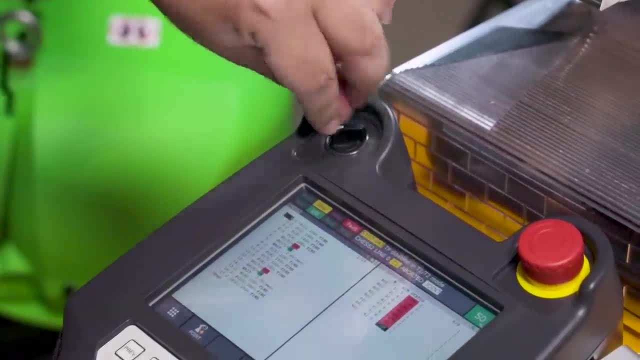 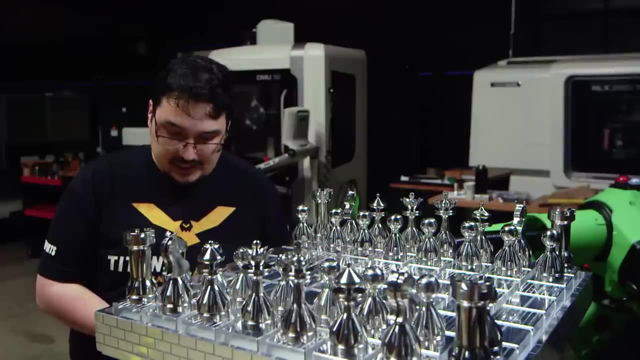 I'm gonna turn my teach pad from on to off And then on the controller, I'm gonna change it from teach mode to auto mode. After we set it to auto mode, the last thing I'm gonna do is I'm gonna take it out of step mode.